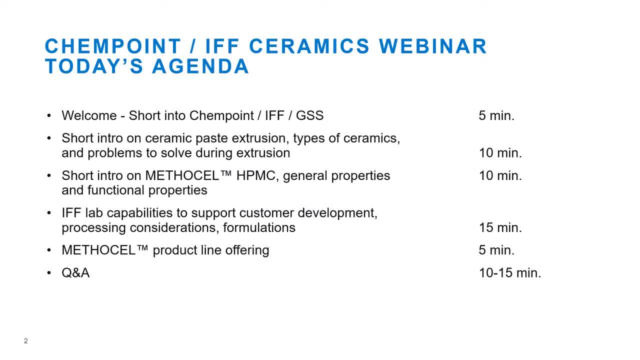 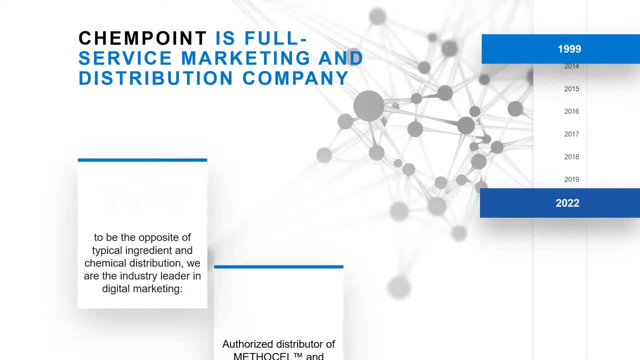 offering that is relevant for ceramic extrusion. We'll leave time for some question and answer. So first start with ChemPoint. ChemPoint is a full-service marketing and distribution company that was founded in 1999.. To be kind of the opposite of a typical distribution. 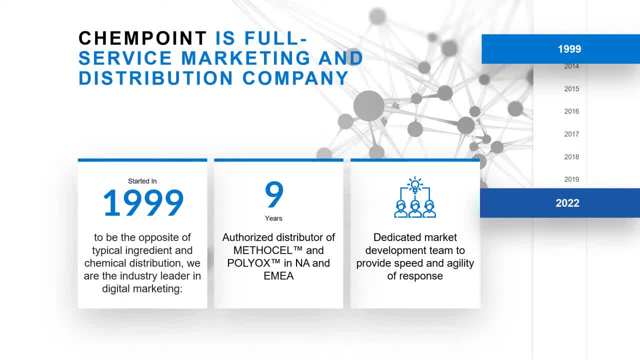 model. we've been the authorized distributor for Methacel and Polyox in North America and EMEA for nine years and we have a dedicated market development team to provide speed and agility of response. And with that I can hand it off to Lindsay to talk more about. 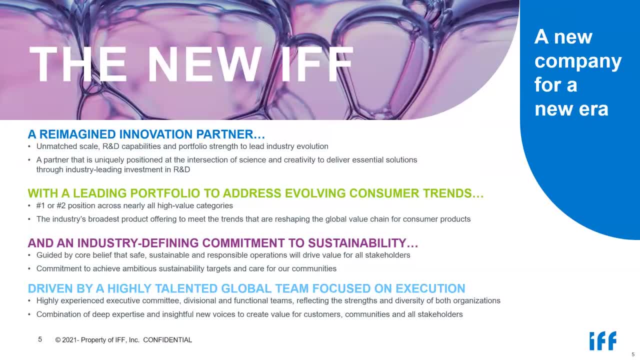 IFF: Lindsay Torreira- Super. Thank you so much, Roland. I'm going to hand it back over to you. Thank you so much, Jeff, and thanks for everyone for being here to join the presentation today. We will get to it in a minute, but I wanted to give a quick introduction of IFF, since 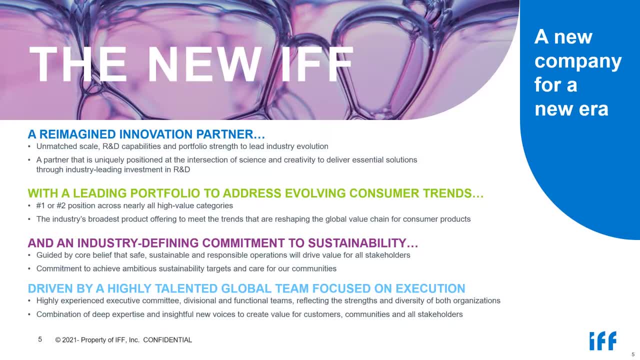 it's likely a new name, potentially for some of you. IFF has a really storied legacy, more than 100-year-old company, But about a year ago we launched the new IFF, which is really a combination and a merger of IFF and the nutrition and biosciences business of DuPont. 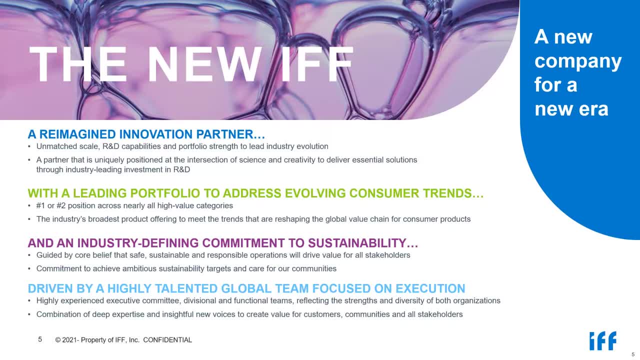 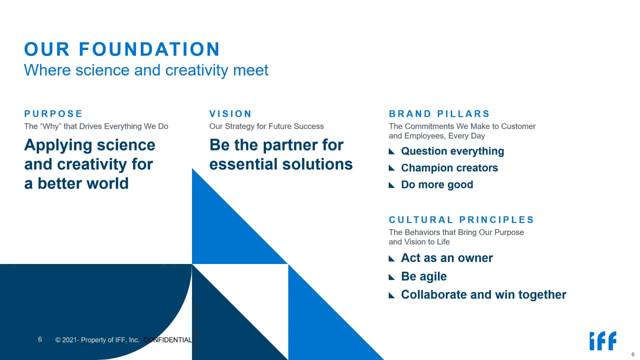 And we're going to be using the IFF as a starting point to really create a leading ingredient solution provider across a wide variety of consumer-oriented markets and with revenues totaling about $12 billion. So our vision and our purpose for the company is really quite simple: It's about applying science and creativity to create a better 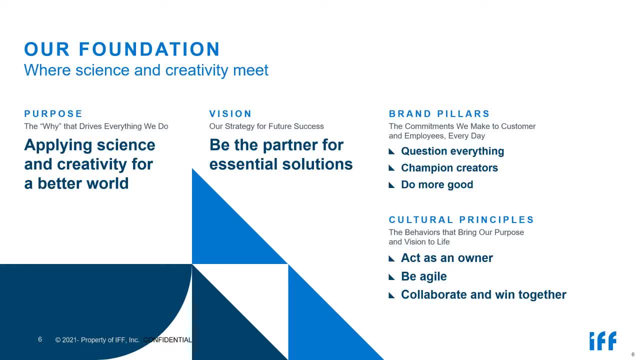 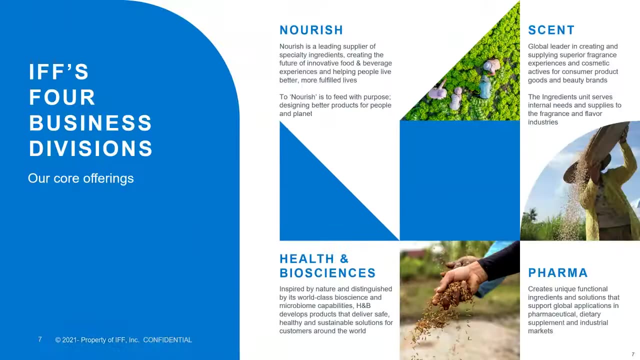 world really, with a very strong R&D pipeline, deep technical expertise, focus on quality portfolio. It's about partnering with customers across those industries to bring them the solutions that they need. The company is divided into four different divisions, As you'll see here. 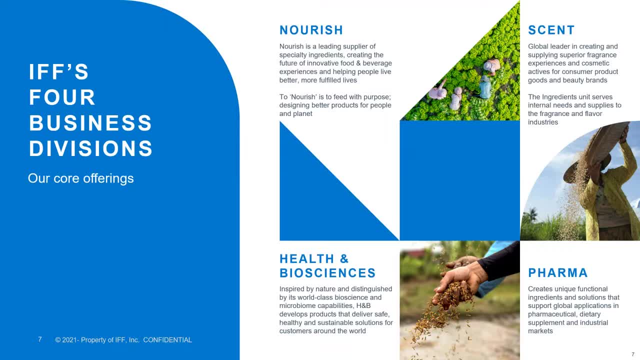 Nourish is mostly focused on food and beverage. We have Scent. that has really an interesting portfolio in the Scent category- Health and Biosciences- really a unique combination from cultures to enzymes, to probiotics and also a pharma solutions portfolio that not only touches 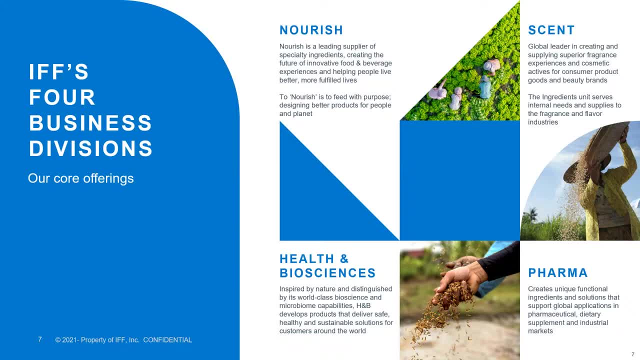 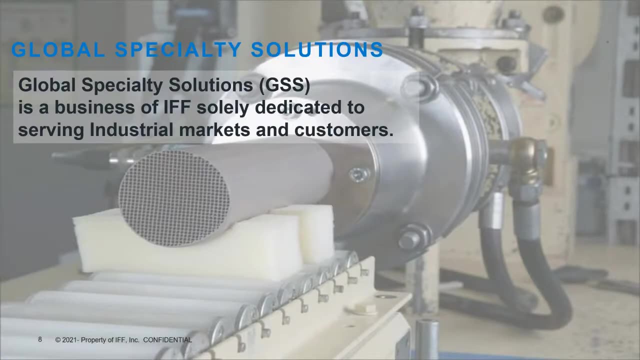 pharma and adjacent spaces, but also some industrial markets as well, which is what we're here to talk about today. So pleased to introduce. Global Specialty Solutions is the business that is serving these industries. solely dedicated to industrial markets and customers, We have our own sales and marketing team. 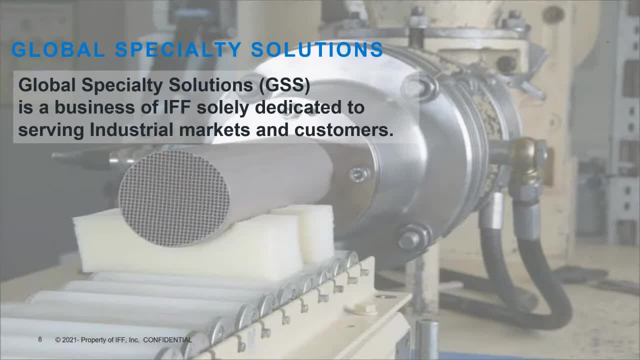 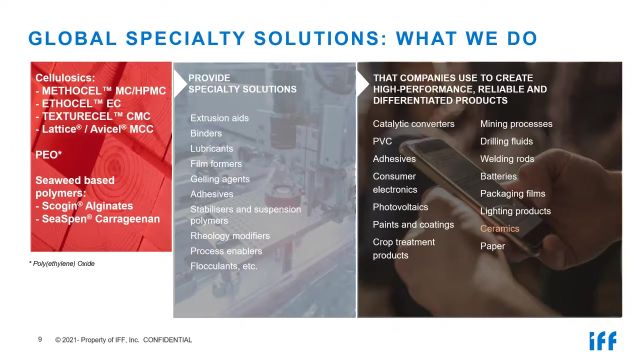 and partners like ChemPoint, and also a deep technical group that supports solely again in the industrial market. A bit about who we are and where we serve. You'll see on this next slide a really diverse portfolio, really broad in the capabilities that we deliver and the functionality. 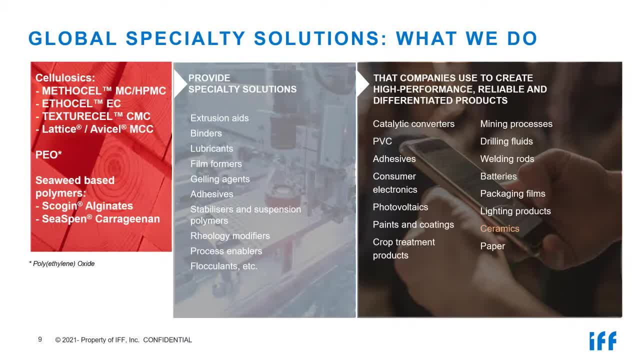 that these products deliver, And on the right-hand side, you'll see just how wide-ranging the applications and the industries that we serve in industrial markets are. There's a list of a few of the key stakeholders that are in this area, So please join me in the Q&A for one moment as we go through some of the main issues. 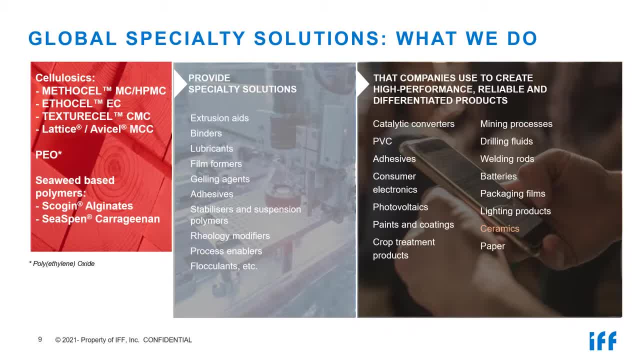 And then we're going to move forward with our final question and answer session. So most of the questions we're going to do today we're going to be asked in the Q&A session right now, And I'm sure many of you are not aware, but I do hope that this is. 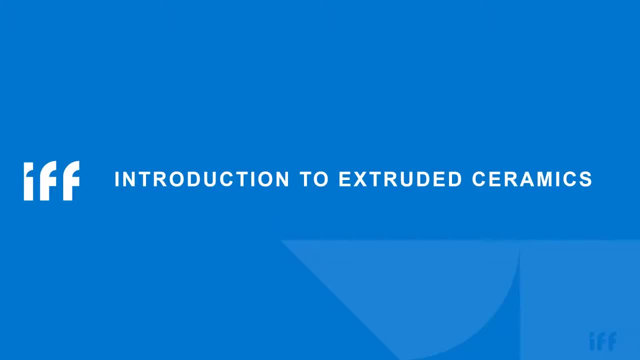 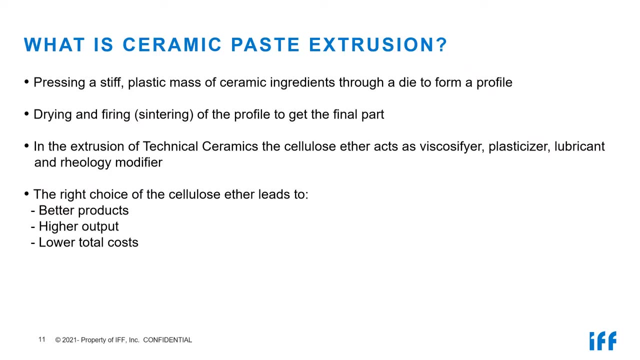 something that will move forward, And we also have a set of questions that are coming up for us in just about any other panel. So let me just notify you that we're going to turn and I'm not going to get too busy with this, I'll just go to the bottom left for just things. 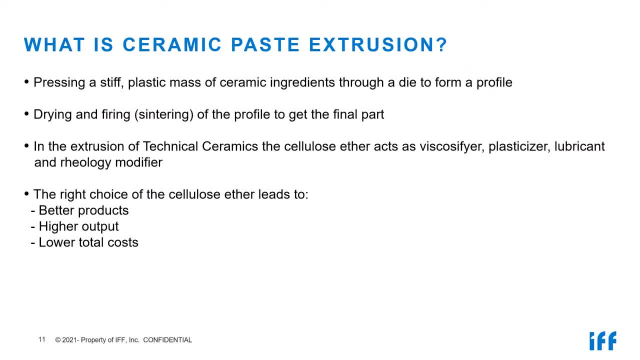 that I'm going to talk about. So yeah, that's how we do it. I'll be sending out the questions. field of technical ceramic paste extrusion. Let me start with the explanation what we are talking about and what not. So we are talking about the pressing of a stiff plastic. 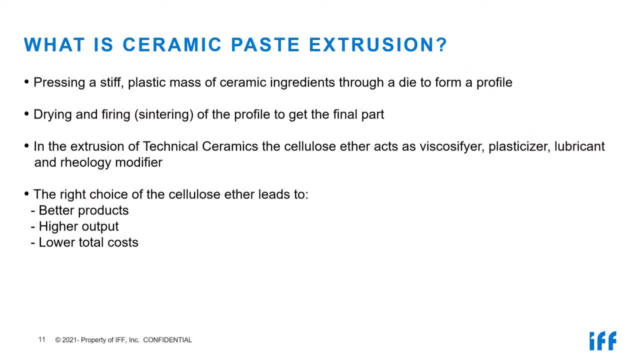 and always aqueous- mass of ceramic ingredients through a dye to form any kind of profile. We are not talking about clay extrusion. Clay is, as you will know, self-lubricating, but it's not used in the extrusion of technical ceramics. Also, we do not talk about thermoplastic. 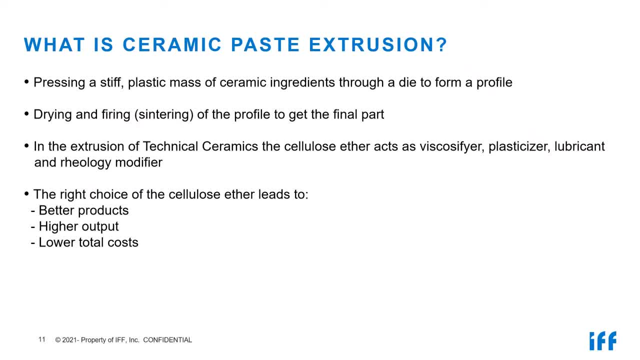 extrusion of ceramics. We are just talking about aqueous paste extrusion. After the extrusion step, normally a drying step of the profile is required, followed by firing and sintering of the profile And of course, in such a typical recipe, a cellulose ethyl is always a big contributor. 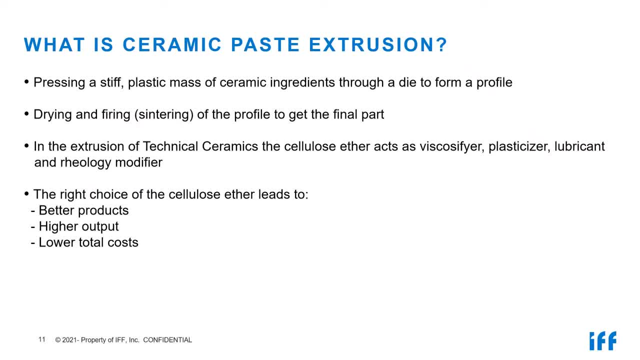 for the processing, but also for the final properties. This is not always so well known, but I will give you some more insight. Cellulose ethyl acts as a viscose filer. Cellulose ethyl acts as a viscose filer. 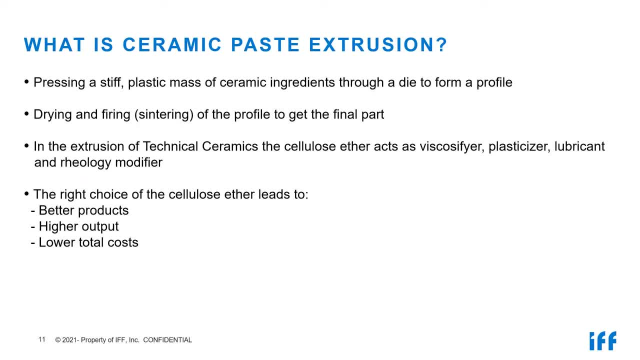 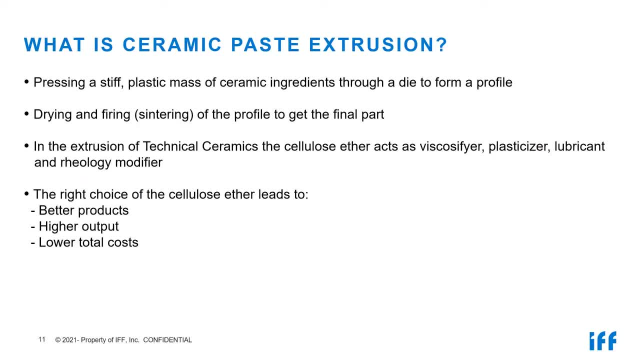 raw materials or maybe also your machinery. This is, of course, something you may be, you might be familiar with, but if you optimize also your additive components, additive composition, mainly the cellulose eater- you really can get better products. and I'm talking 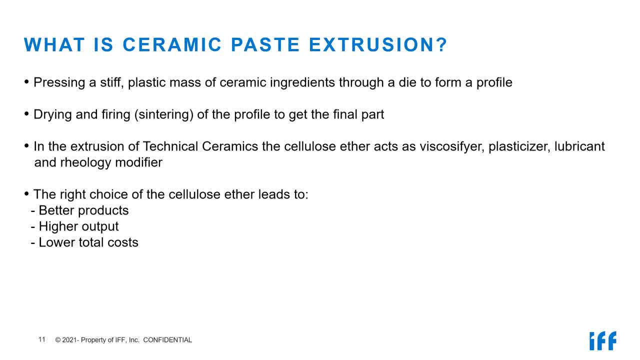 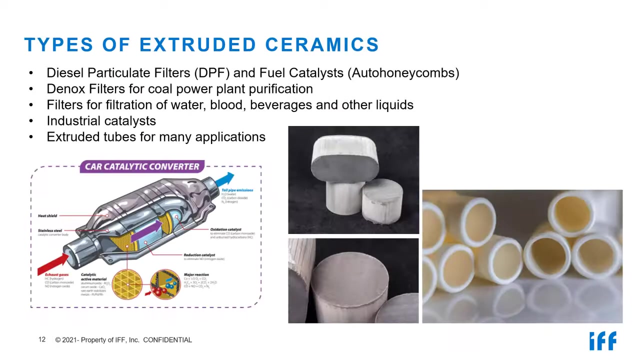 about better end products, higher output- in many cases up to duplicated processing speed- and lower total cost. lower total costs, for instance, can mean a significantly reduced off spec rate, and this is, of course, a question of profitability. next slide, please. there are many types of extruded ceramics in the market, and if you drive a car, you definitely will. 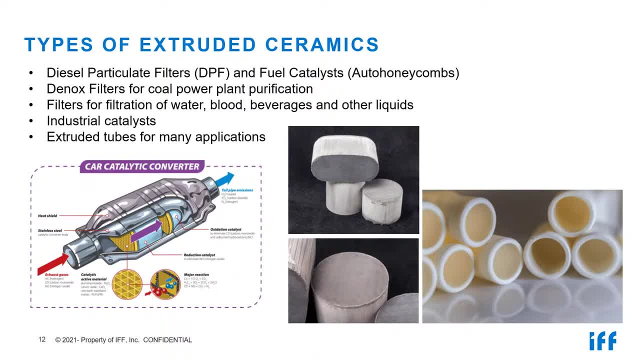 have seen or you will have used some of them, like diesel particulate filters or fuel catalysts, which are everywhere installed in cars, excepting you are driving an electrical vehicle. also also very well known and a quite big market are denox filters, which are used in coal power plant. 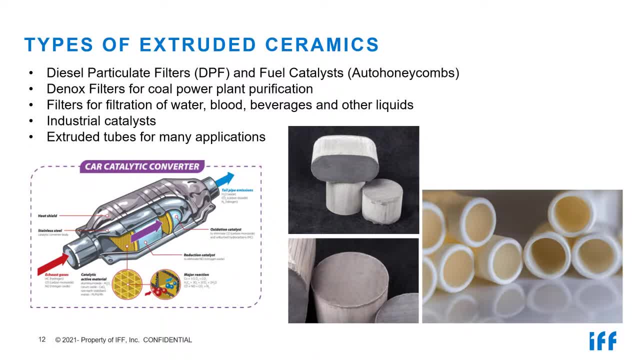 purification processes and not so easily to seen for the end user is the filtration of many liquids. beverages, water, blood and many other liquids are filtered through ceramic filters. they all are extruded for the chemical industry, especially for the oil industry and oil processing industry. industrial catalysts are 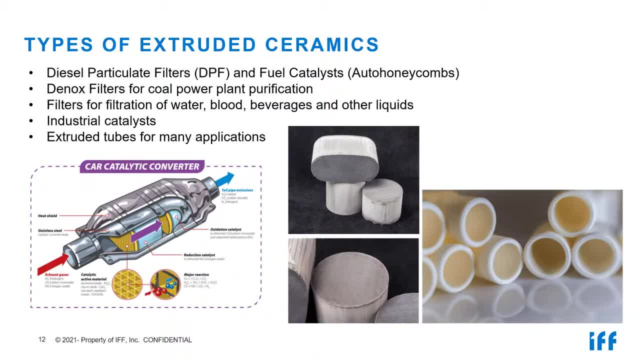 very essential, and many of them are made out of ceramics or are being extruded in ceramic form. and finally, there's a one more market which I would like to mention: extruded tubes for many applications, and here, in this case, I would like to mention especially silicon carbide and alumina tubes, which are quite often used in high temperature applications. 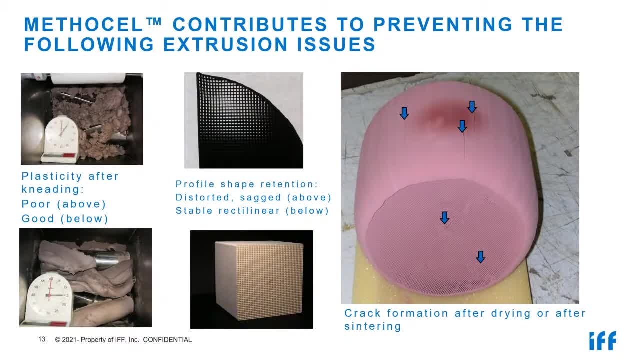 next slide, please. so this sounds very quick and easily done. you just make a paste and you press it through a die and, just by good luck, you get a nice profile. but that's only half of the truth. it's a little bit more difficult and besides all those research papers, there shouldn't be technical issues. 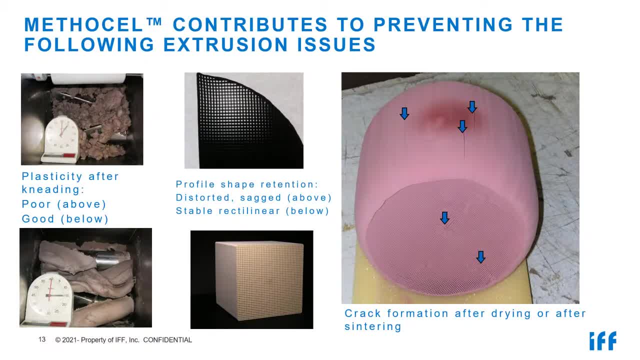 the enthusiasm normally you have easy. you quickly get the experience of some problems and some of these problems you can solve by the right choice of the additives. i'm talking about, of course, about the metaset additive. let me give you some example. a major issue in extrusion starts already very 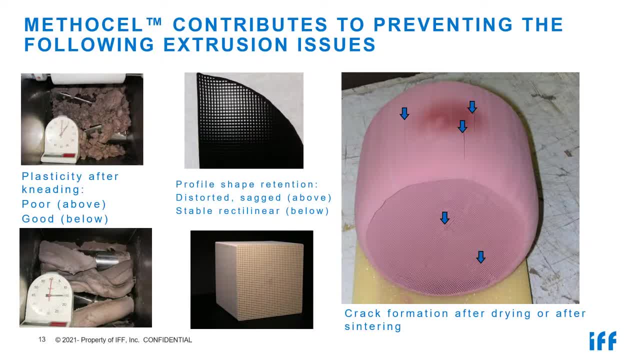 early in the process when you make your paste. the plasticity of your paste is significantly contributing to a well done or poor processing. here in the left corner you can see. you can see two pictures. the upper one shows a ceramic paste with very poor plasticity and the lower one shows 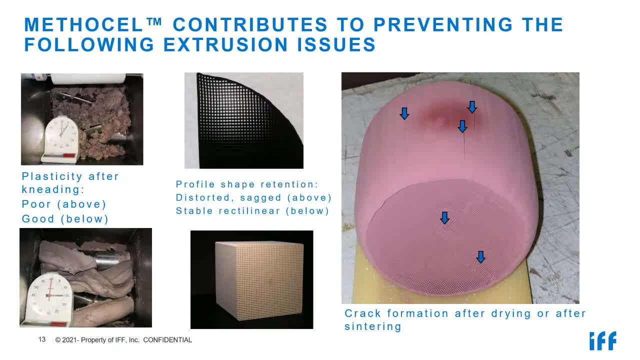 the same formulation with a very nice plasticity. now you will believe i it's just a question of time: how long you need, and as longer as better. in many cases you are right, but i have seen cases where even after um needing of several hours, you still have these little dumplings, like in the upper picture on the left. 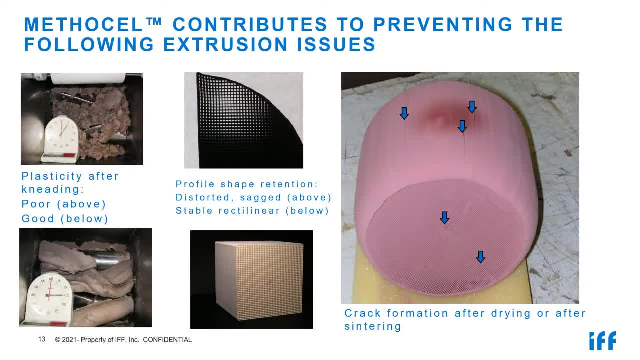 so the plasticity did not increase. but with the right choice of cellulose ether it is easily done and you get a mess like it can be seen on the picture below. a second problem, typical problem is the so-called shape retention. shape retention of your profile especially has a high 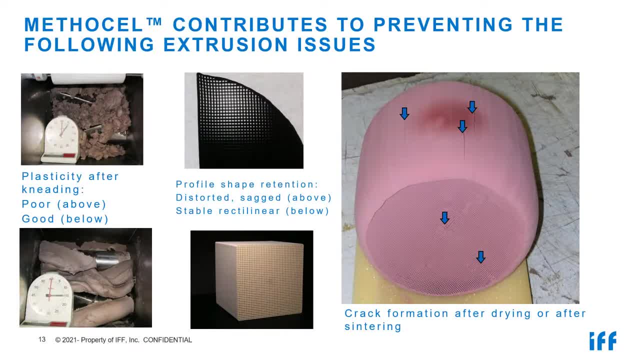 importance when you extrude hollow profiles like honeycombs. in the upper picture you can see a picture of of a shape retention problem. in this case it was extrusion of silicone carbide to a hollow profile, of course in honeycomb. as you can see in the upper part of the picture some segments. 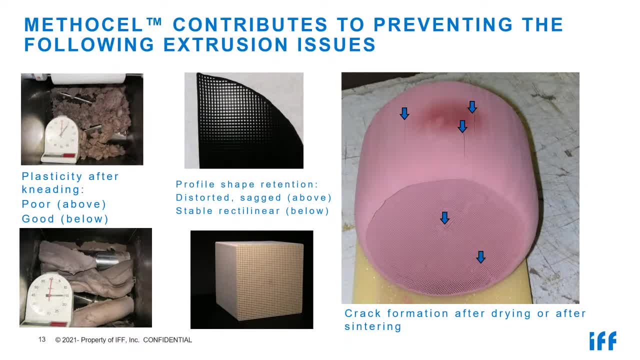 collapsed, a little bit at least. they are distorted and sacked and this is of spec. you cannot sell away to a customer. um, silicon carbide is expensive. they reduce the distribution of the notice. it is a low-tech process. you cannot love the quality of this particular product and this is what was shown. in the upper part of the picture. some segments collapsed a little bit at least. they are distorted insect and this is off spec. you cannot sell away to a customer. um, silicone carbide is expensive. this is reduced for long term use of this is, of course, not suitable for as many the price range, but it is really. 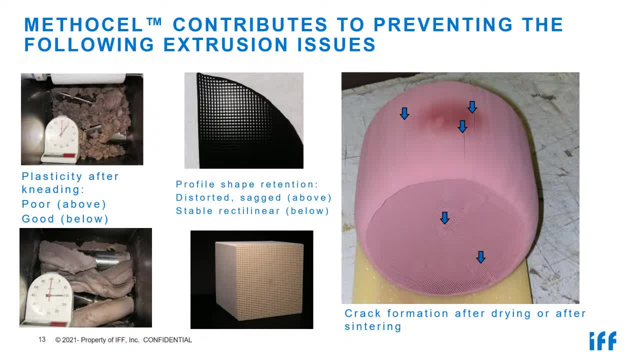 your production speed and leads to off spec, which is costly. what you like to get is a stable rectilinear structure, as you can see in the picture below, and cellulose eta definitely contributes to the solution of such issues. now we are coming to a major issue: crack formation. 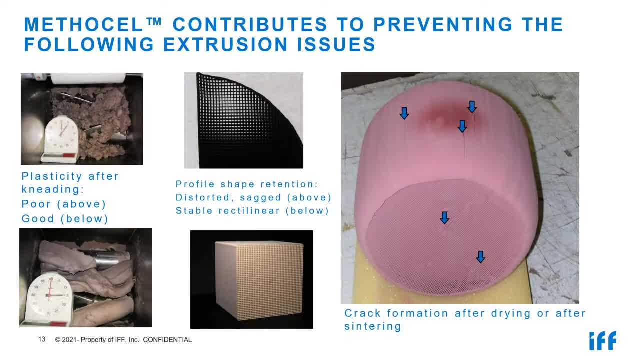 i'm quite sure there's nobody here in the line who never saw track formation during extrusion. it can happen at many um at many places and it can have many reasons. in some cases the right choice of metal cell can really help and can heal a problem or can solve a problem even um. 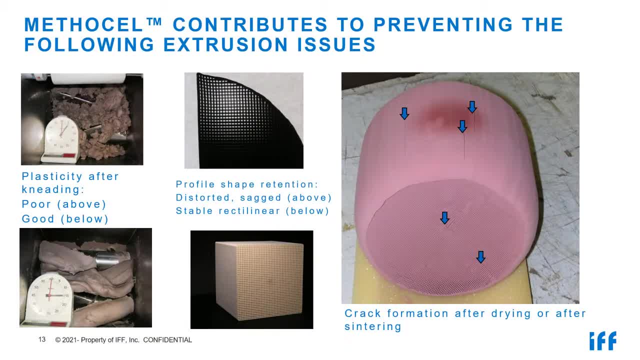 even if the metal cell is not the reason of it. so, for instance, um typical reasons for crack formation are wrong batch processing, wrong mixing. uneven distribution of water in the batch can be. it can has to do with so simple things like cutting the profile after the extrusion step. 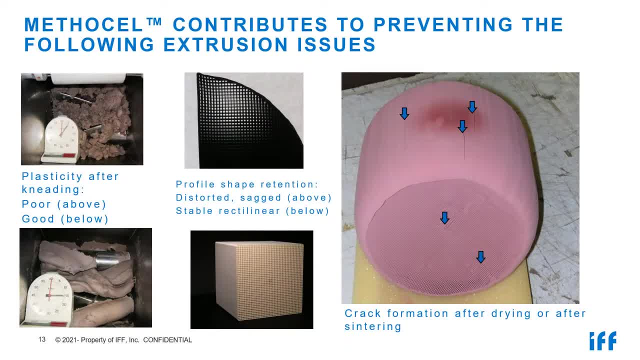 with handling the profile into the drying room, with the drying room conditions we see air distribution in the drying rooms, with calcination conditions and so on and so on. there are many, many contributing parts, but cellulose eater, in some cases at least, is able to solve some issues which you cannot solve with any other tools. 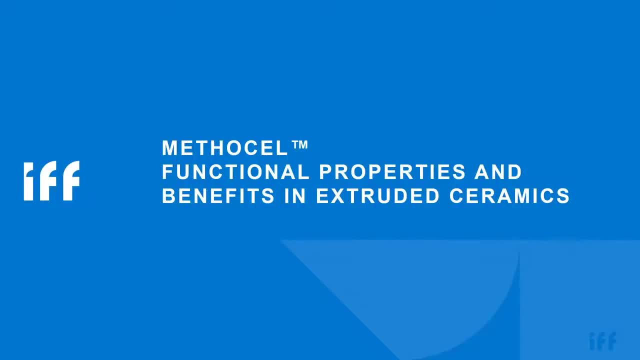 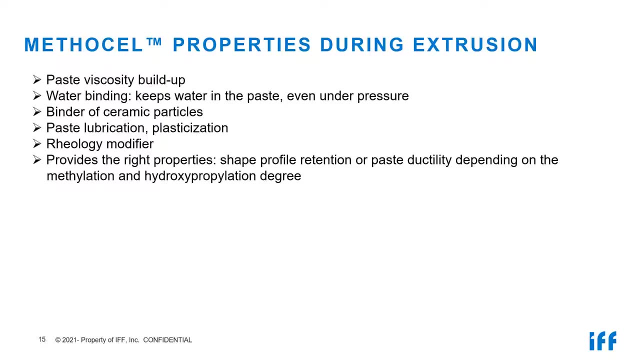 next slide. please now let me come to the functional properties and benefits of metal cell in the extruded ceramics. so, as i said already, main, main visible effect is of course a viscosity build up in the paste and not so obvious but extremely important is the wine water binding force. um, i said already, 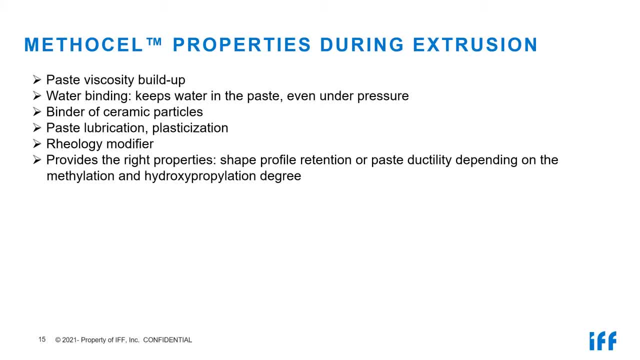 metal cell is a binder, but it is also a binder for the water. it keeps the water in the paste, even under high pressure. sounds unimportant, but it is of a very high importance if you ever have seen a water drop falling out of your machine, for instance at a seal or 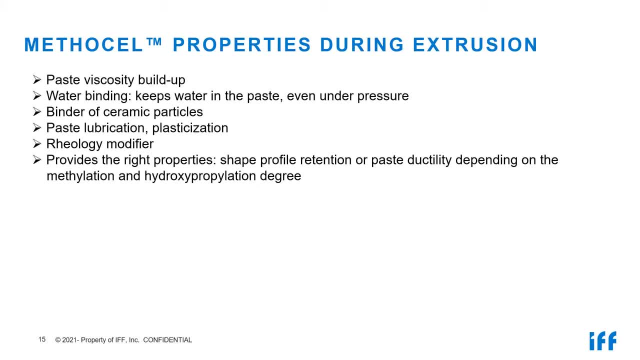 some other parts. this can lead to extremely fast development of pressure and to a high danger for the machinery. machineries even with one centimeter thick steel can break, and this is a question of the water retention capability of the of the cellulose eater and definitely this is here's. 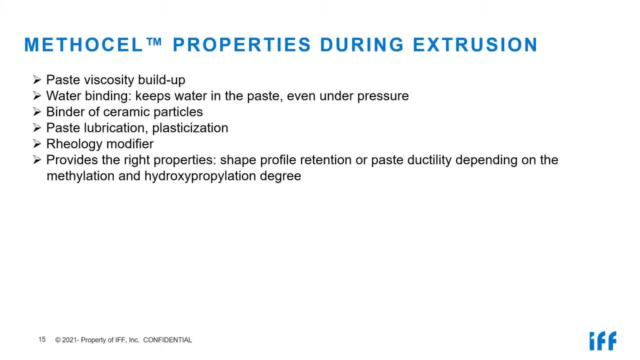 a contributor in such a problem. if you have ever seen such a problem, please immediately replace this cellulose eater or reformulate it. it binds the ceramic particles, it lubricates the paste and plasticizes it. it acts as a rheology modifier. as i said already, there are many different possible rheologies you can choose. 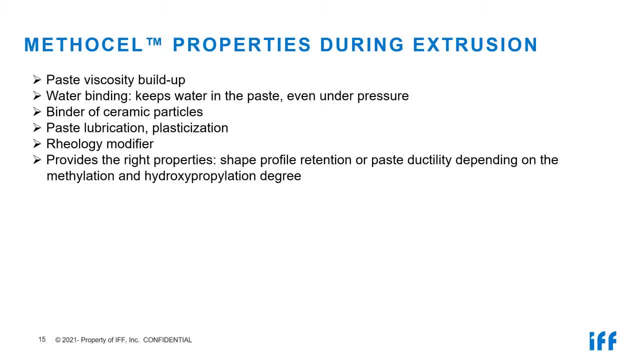 from newtonian to pseudoplastic, and there are many other details we can discuss offline if you like. and of course, i want also to address the topic of shape retention and paste ductility. both are impacted heavily by the substitution of the cellulose chain, which means 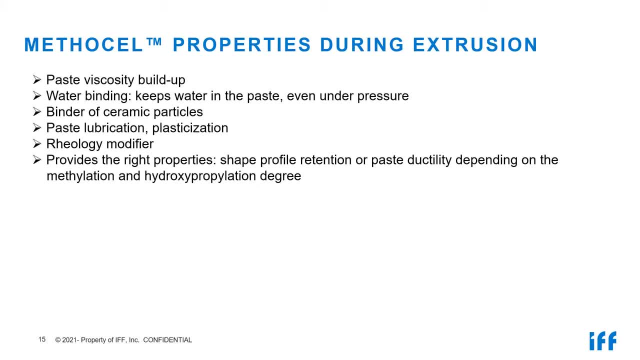 translated into, let's say, normal words, it's: it is depending on the so-called chemistry of the cell around the concrete terms, and this is exactly why we are looking at different conditions in order to find the most optimal for your metal cell. so there are grades where the paste ductility. 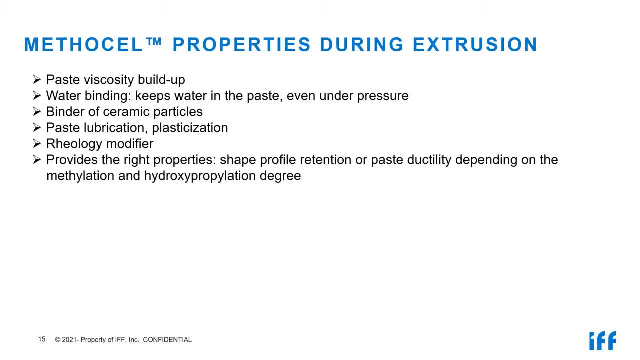 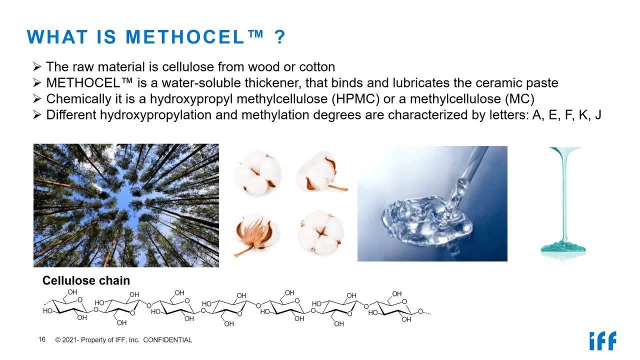 is high and there are grades where the paste ductility normally is lower, then the stiffness is higher. it has advantages and disadvantages, so it is always a question to find the optimum for your recipe and what your individual conditions really require. next slide, please. derived from nature, our main raw material is wood cellulose from wood or cotton and after a very 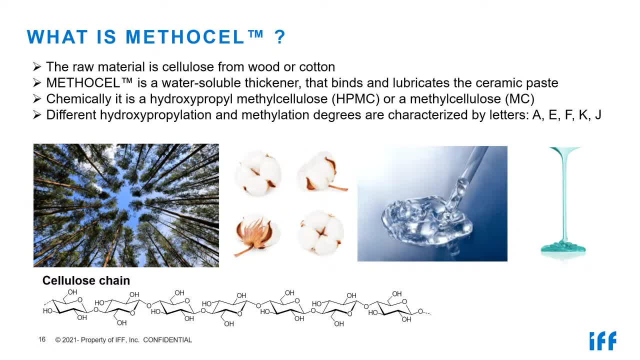 complex processing in a high pressure reactor reactor. at the end we get white powder which is water soluble and binds and lubricates a ceramic paste. chemically seen, it is a hpmc- hydroxy propyl metal cellulose- or an mc which is a metal cellulose. these are two different classes. 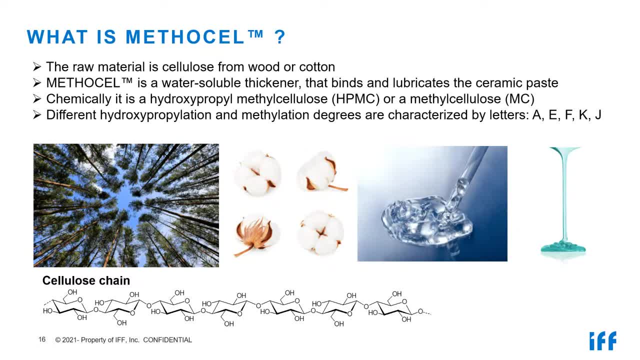 and to. in order to characterize them a little bit easier, they received. these classes received letters, so we have a metal cell a class- this is a pure metal cellulose- and several hpmc classes- metal cell e, f, k and j. at the end of the. well, please go back. yeah, thank you. at the end of the slide you can see a segment of a cellulose. 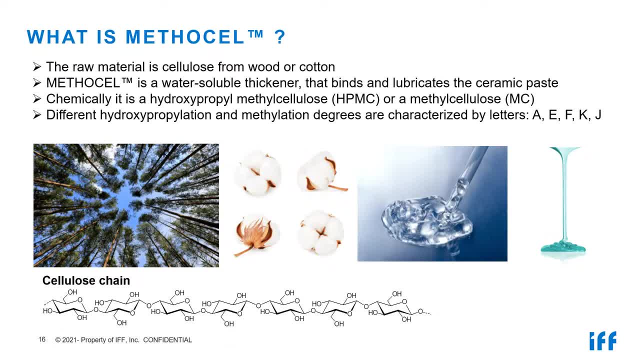 chain and you will easily see. there are repeating units, so-called glucose units, and every repeating glucose unit has three free hydroxyl groups and this is where we make our reaction process, where we can test if there are any elements of a cellulose that we 하는데 in, called motility. 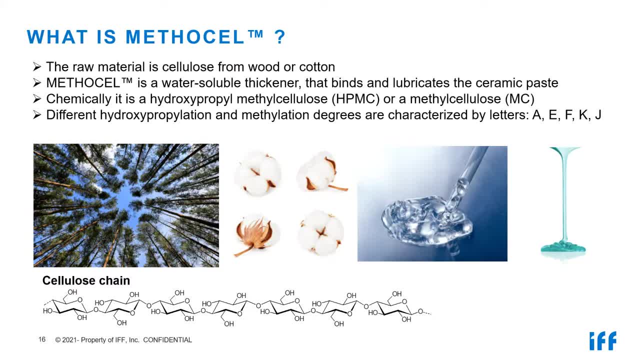 if, if there that here on the left were very specific, only organ LGB equaled to the normal proposition for identifying the microfiber and in our cellulose pair there are a few different regions. again with this we can consider that there are other promotion areas that are. 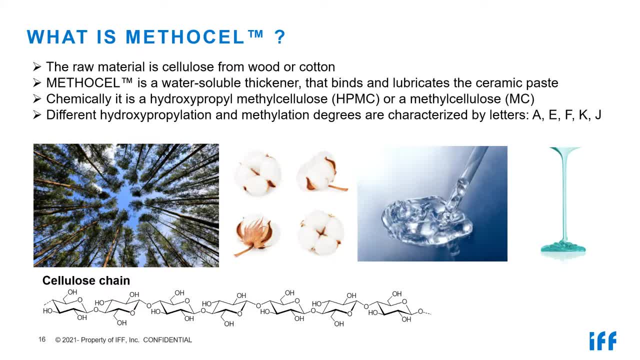 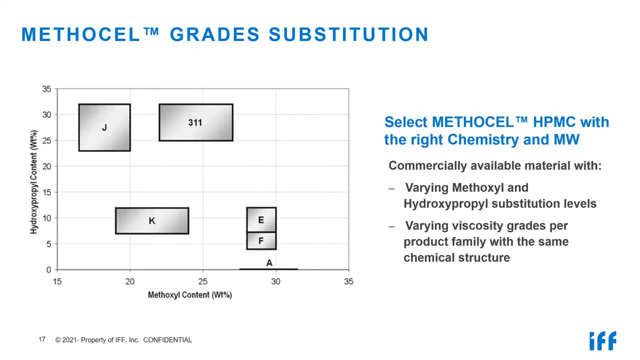 in Portal onto the 1. here there is a molecule that also has, at this phenomenon- example of cells- this choice of parameters. next slide: yes, if you look now, if you, if you make a graph presenting the metoxylation content and the hydroxypropylation content. 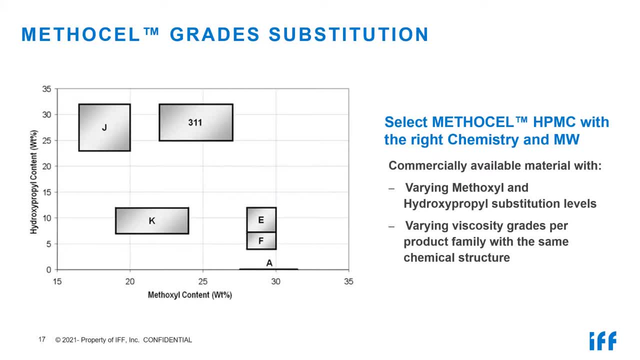 on the two axes you will get some boxes and these boxes represent the specification windows of our cellulose eaters and you can see very below there is also the a class, but it is just a line, it's not a box, and the reason i said already metal cell a is a pure metal cellulose. 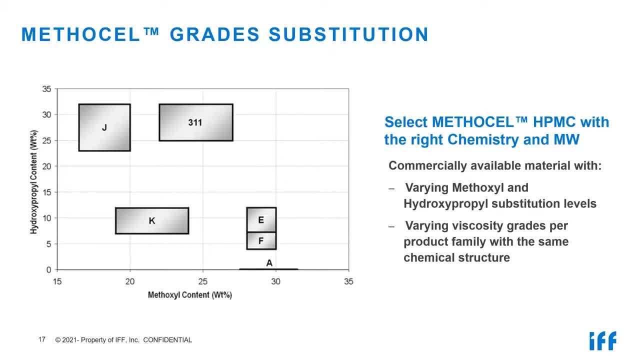 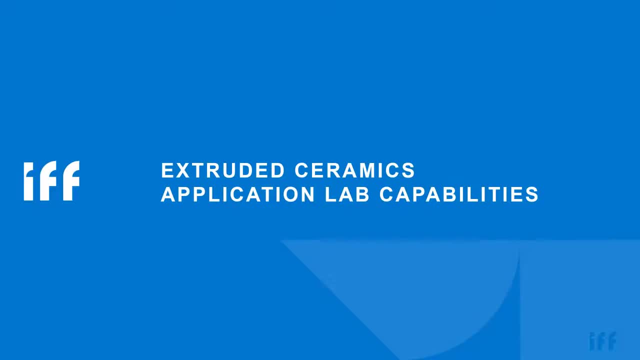 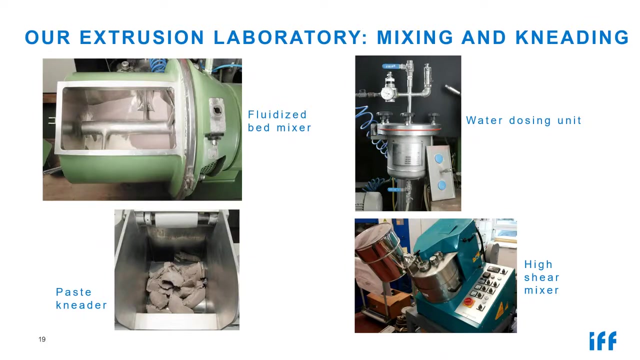 and, of course, hydroxypropylation content is zero. that's the reason why it is just a line next slide. yeah, in order to support you in your development work, but also in order to produce lots of data, to get experiences with ceramic formulations and in order to develop better products, we have established a ceramic extrusion. 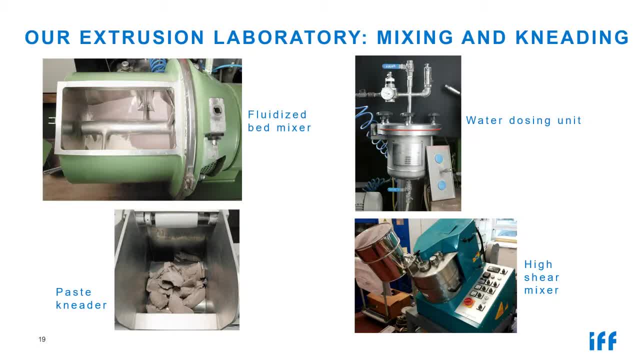 laboratory already 25 years ago. some pictures from our lab are shown here. on the first slide, left above a fluidized bed mixer which we are using for the dry mix. this is the only way to get a homogeneous dry mix between heavy powders, heavy particles like silicon carbide or even 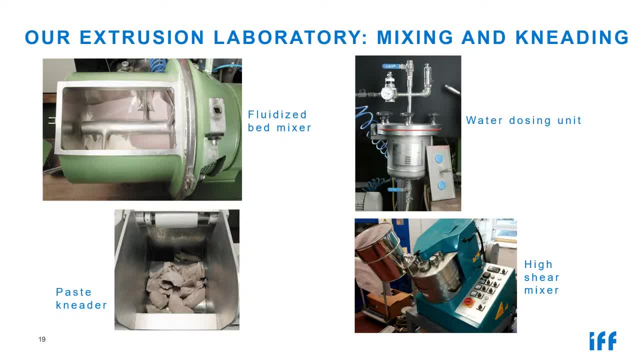 yes, there are many others, zirconia, for instance, and light particles, for instance, cellulose eater. yeah, if you have a slowly running mixer, you never will get a homogeneous distribution, and this is, by the way, one of the reasons on of the reasons for a later crack formation later on, um, after you have. 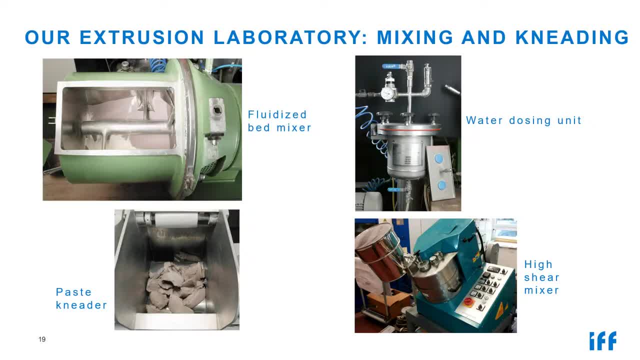 a received a homogeneous dry mix, you spray water in and the process is ended when you get small dumplings, very small dumplings, which you empty out of this container and fill into a paste needle, which you can see left below. this is a typical needle, uh, which further plasticizes this container. 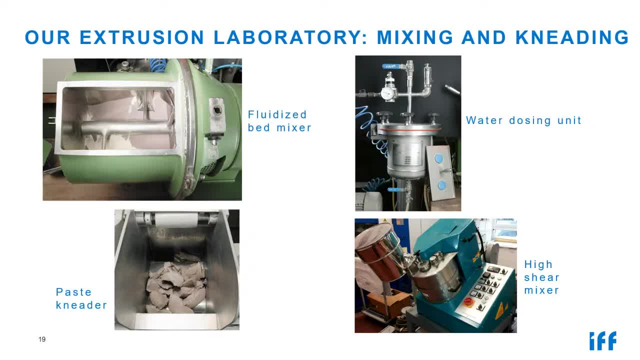 it will build the mass of the medicine and also, as a result, it will be able to absorb more particles from this tube into the body and it will use this into the mass of the treatment, the mass before you enter you, before you put them into the extruder, our water dosing unit. you can see. 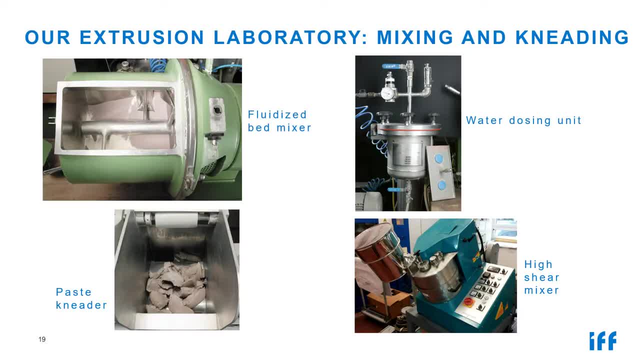 right above. this is a simple equipment, but very useful and precise. what i showed you is a two-step process. step For that you have to look to the picture right below. This is a Heiche mixer, a so-called Eirich mixer, which is a totally different technology. It works in one step and I think 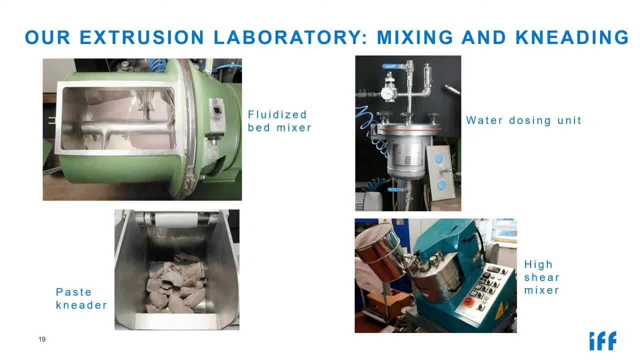 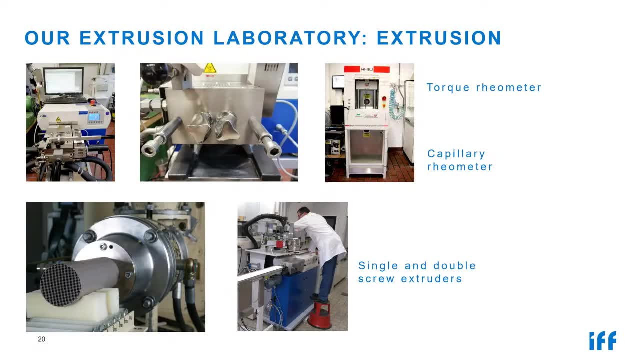 in most cases you can get very similar results. Next slide: Okay, now we have received the paste. and what now doing with the paste? The first is not to make an extrusion test, but first to test the properties of this material. For that, 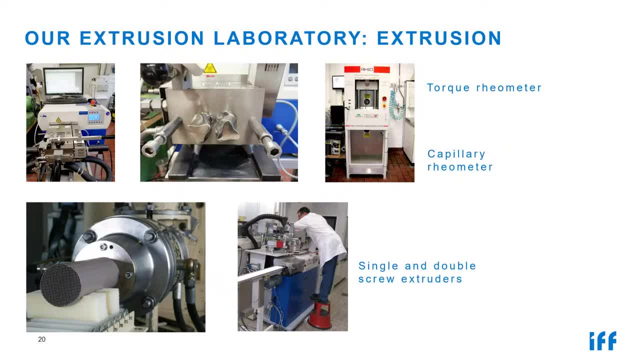 please have a look to the two pictures left above. in the first line We are using a torque rheometer from Brabender, which is nothing else than a small kneading chamber with two kneading pedals, which you can see in the middle picture. But they have in this kneading 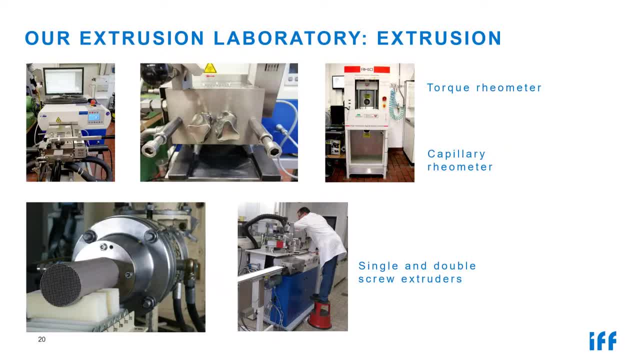 chamber there is a torque sensor And this is the first test. This torque sensor indicates very precisely where the relation starts, because at the point of the relation of the cellulose ether in the ceramic paste your torque will rise up. In an extrusion test, your pressure would rise up. 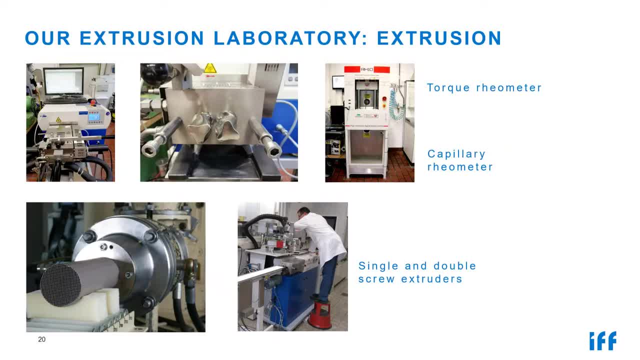 The next picture shows our capillary rheometer, which we misuse as a piston extruder. So it is a piston extruder, and then in the lower line you can see our single screw extruder. This is an 8 cm machine and a double screw extruder which we are using as well. Next, 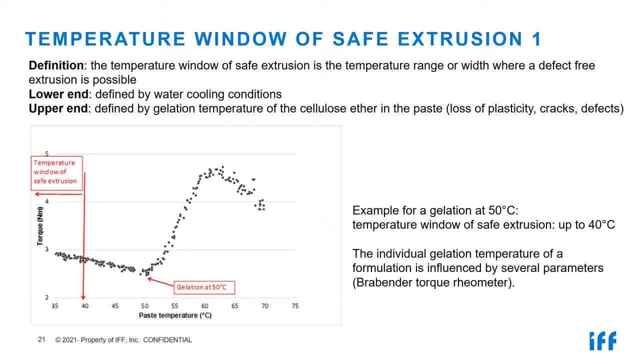 slide. So now we are coming to a very big and important topic which leads to a serious understanding of every individual thing. So what we are doing here is to create an external test. What we are going to do now is to test theоstole himself To�� will test out the cellulose ether. 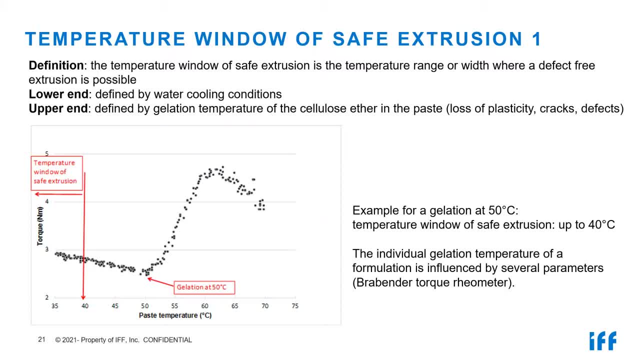 individual paste you are formulating. i mentioned already that a limit of all extrusions is the isolation of the cellulose eater. this is a very unusual property. normally if you heat up a solution of any ingredient, let's say sugar or salt, the solubility increases with the temperature. but 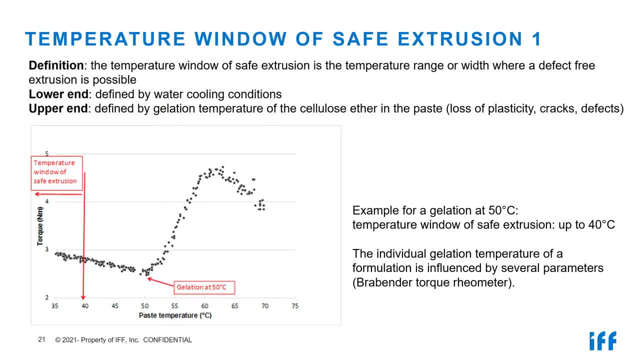 here. in the case of cellulose eater, it's exactly in the opposite direction. at a certain temperature, the solubility is decreased and the cellulose eater starts to flocculate out of your solution. and if this happens in a ceramic paste, you can't see it anymore because of the invisibility. 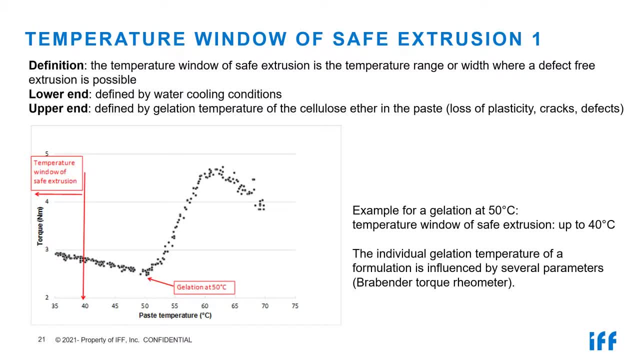 invisibility of the ceramic particles. but it happens and this is a high danger of your extrusion process and that's the reason why we have made a lot of work on this topic to to enable you a safe extrusion, especially for your plant. it is of importance because you do not have 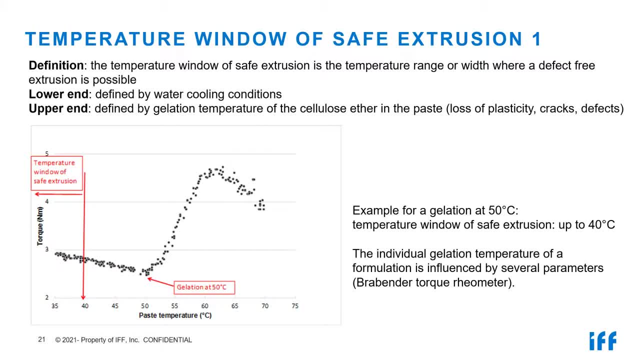 such a nice temperature control in your plant like in the lab, at least in most cases. yeah, we defined a so-called temperature window of safe extrusion- extrusion where you can safely run your extrusion process also under plant conditions, and we define this safe window to be 10 degrees below the relation temperature, where the relation 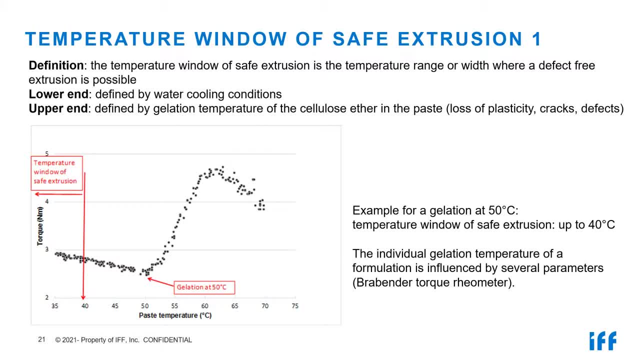 temperature is. you can measure with this torque rheometer trial here in this case. this is just an example. in this case the relation temperature is in the range of 50 centigrade and this means the safe window of operation ends at 40 degrees. now your question is um. 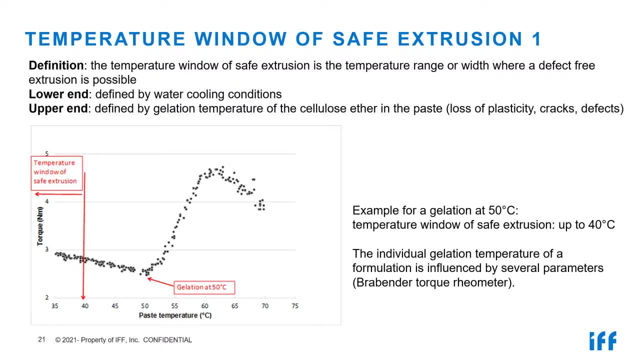 this is 40 degrees. um, yeah, maybe this is not a large space. yeah, you might be right. then please enlarge the space. there are different possibilities. you? um, we have a toolbox. yeah, it's like in a car repair and by modifying the conditions you can move this relation temperature upwards or downwards, depending on your needs. 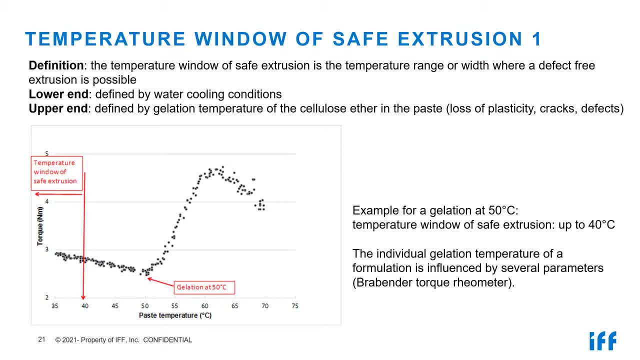 so um, the safe window of extrusion has a lower end, which is, of course, defined by your water cooling conditions. please do not think about your lap in the lap. normally you have a very enormous size control. please think about your plant conditions. this is really the challenge in. 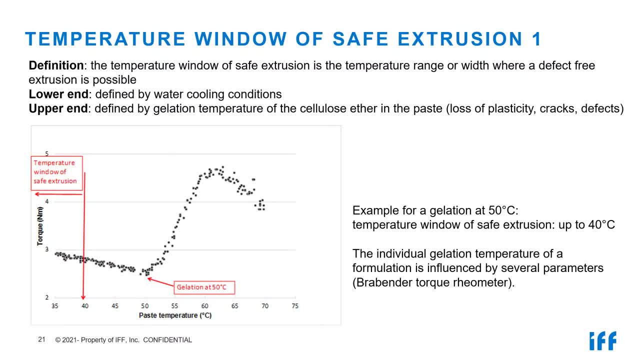 in the plant. you might run your extrusion day and night, 24 hours per day. you might run in winter and in summer. you might face a challenge that the tap water changes the temperature between the seasons and you might face many other challenges. one of them is the extruder in the lab. 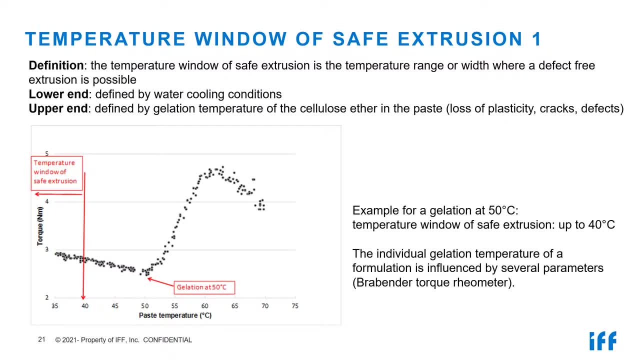 normally is smaller than in the pr in the plant. if extruder is large in the plant, of course the cooling conditions are worse compared to the lab because the um, the ratio between the cooling surface and processed material, is very different from the lab and normally it is a negative effect which leads to an increase of 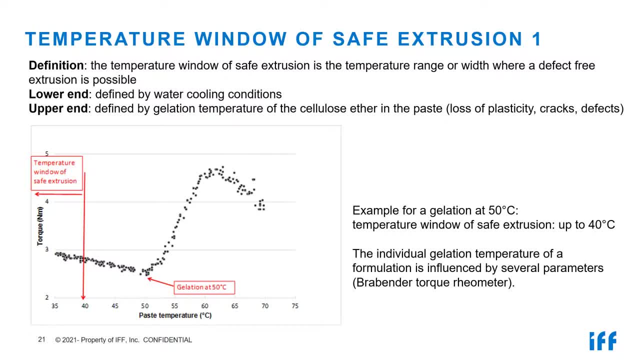 of temperature in the processed paste. this means you are reaching, you are coming closer to the relation temperature compared to a similar trial in the lab. so i said the lower end is defined by your water cooling conditions. the upper end, however, is defined by the relation temperature of the cellulose ether in your paste. there are five reasons to influence this relation. 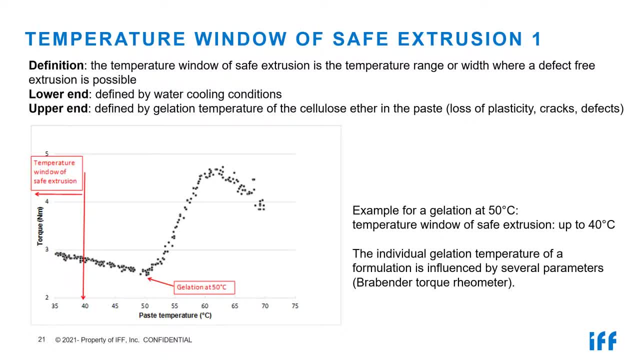 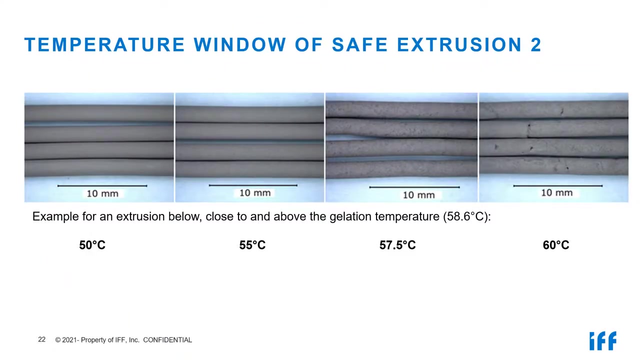 temperature, or five origins which contribute to the relation temperature, and they are very individual, depending on four recipe parameters and one processing parameter. and this is just an example, next slide. this is another very nice example demonstrating how important it is to stay, to stay in a large distance, for in this safe window of operation, so in a certain 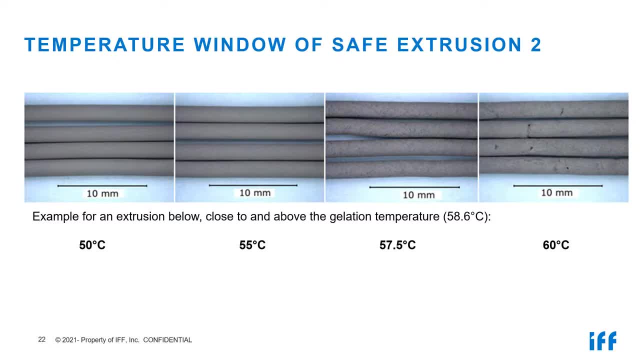 test. in a test batch we measured with our torque rheometer. that's the relation temperature of the cellulose ether in a certain mix was 58.6 centigrade. then we made four extrusion tests at four different temperatures and checked the profile quality. please have a look to the first picture. 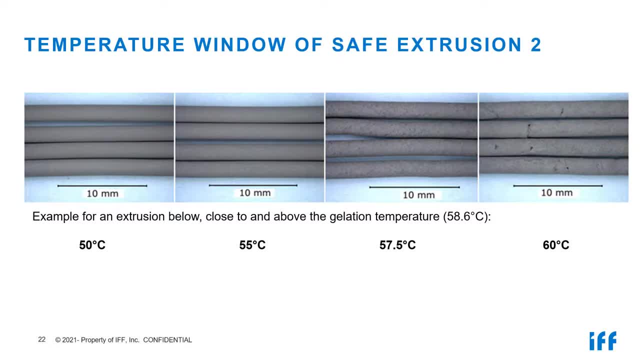 we extruded this material at 50 centigrade, so nearly 10 degrees below the relation temperature. the profile looks very well: no holes, no very smooth surface, everything is okay. but then, five degrees later, five degrees higher- a second picture you can see. the surface shows. 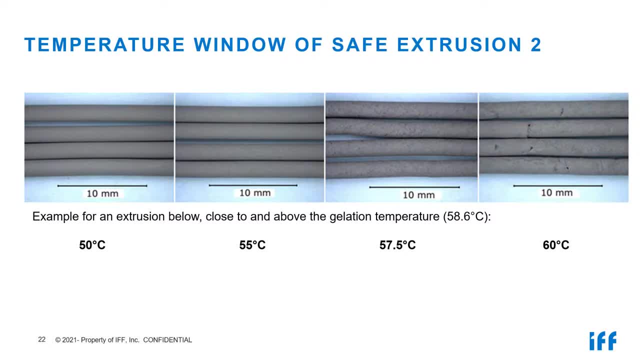 already this slight, slight, slightly cloudiness. um, the profile is still even and looks still okay. but you will realize that first micro defects occur. but maybe you can still sell this material. you should make a test after centering. then picture number three, very significant, you are still one degree below the relation. 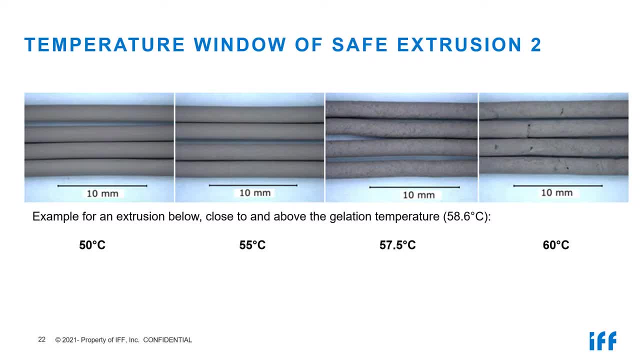 temperature, but you get already a very good result: very coarse and porous structure. deformation of the shape- it was a full profile, not a hollow profile- a hollow profile would look even worse, you can be sure- and smaller pores on the surface. finally, the extrusion test at 60 degree, one more than one degree above the relation temperature. 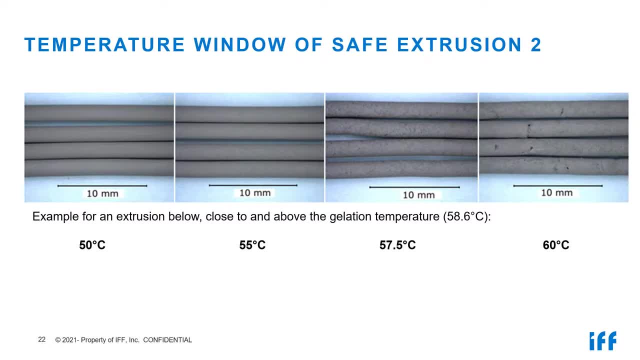 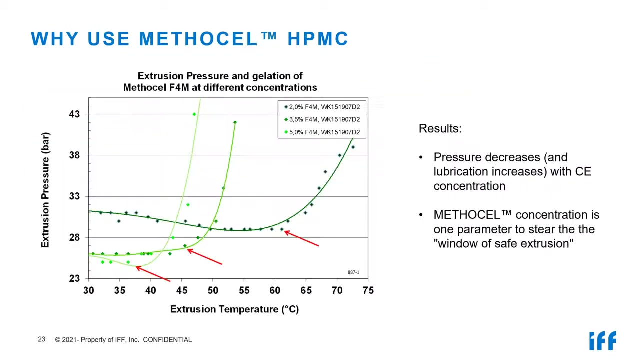 this is a disaster. you never would sell this. definitely. this all is off spec already. extrusion here and in picture three is all defect, definitely yes, this is just for demonstration purposes, to show how important it is to stay away from this relation. temperature. next slide some more examples here to show you the relevance, how to formulate the relevance of. 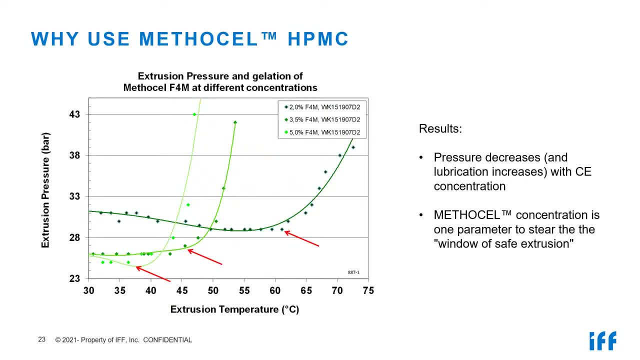 different parameters. in this example we would like to demonstrate the relevance of the concentration of the cellulose eta. yeah, in this example we are using three um metal cell concentrations. in all cases we were using metal cell f4m first test run with two percent in the mix. 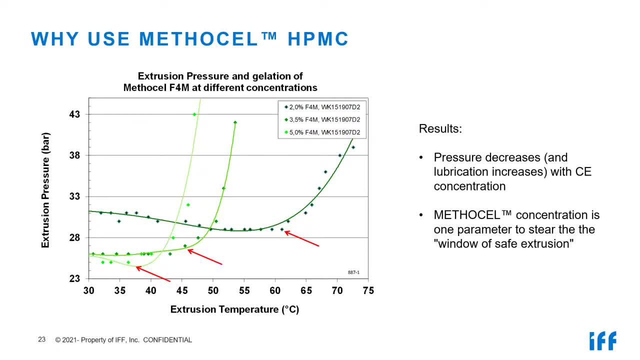 please have a look to the dark green line first. the line shows a slight decrease. this is a normal effect which you observe in every polymer solution. when you heat up polymer solution, normally the viscosity drops. but here, in this case, you are coming to the relation temperature close. 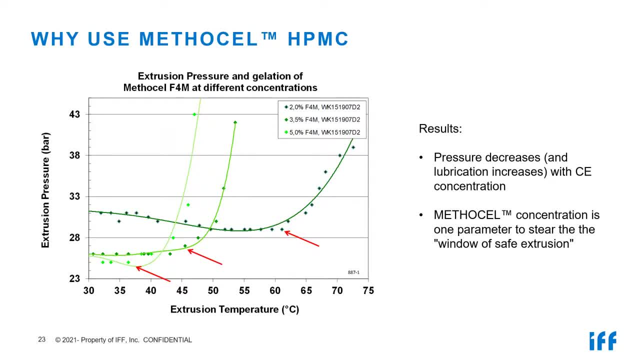 to close to 60 degree, and then there is a sharp rise of the extrusion pressure. and why? because, of course, the cellulose eta flocculates. it's not soluble anymore. if it is not soluble anymore, it cannot contribute to plastification, lubrication and so on, and that's. 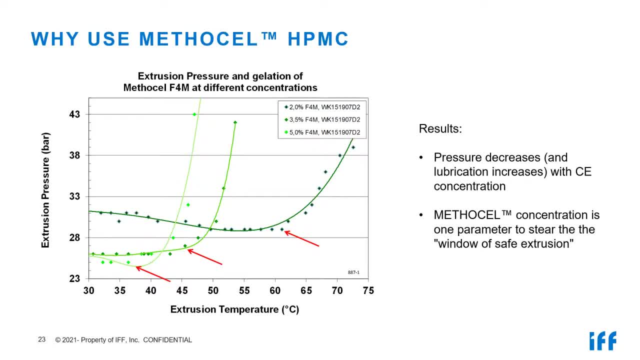 the reason why the pressure is rising. second case with 3.5 percent of f4m. now we are coming to the second line, starting at 6 bars extrusion pressure. you can see, you have, you can see that the extrusion pressure drops significantly. so the lubrication is definitely better. this looks very good. this is 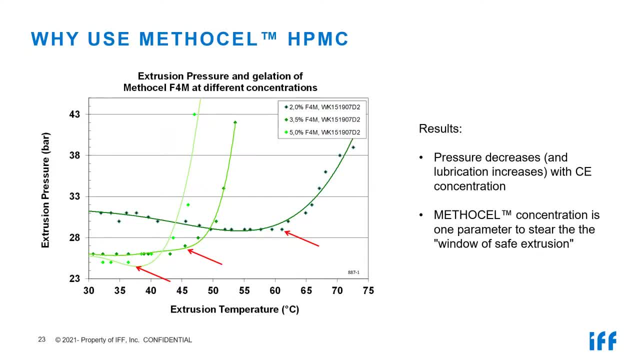 an advantage, but at the same time you get a disadvantage, because the um, because the isolation temperature drops from roughly 60 to down to roughly 45 centigrade centigrade. this means your window of safe operation drops by- is reduced by 15 centigrade. this is a lot. if you have difficulties in cooling, this might be um hard and example. 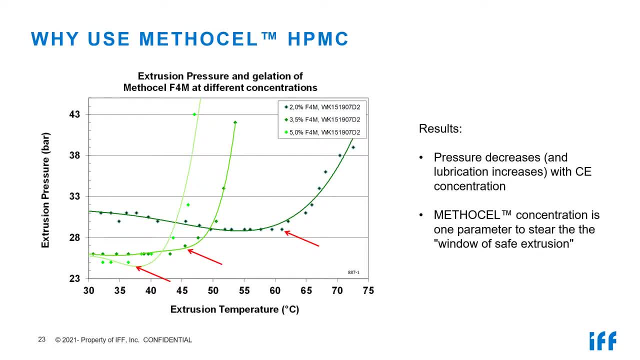 number three: with five percent of f4m um, you can get- still slow, i know- a little drop in the extrusion pressure, but this is not significant, significant anymore um. however, you get also a further drop in the relation temperature and now your window of safe operation is really getting 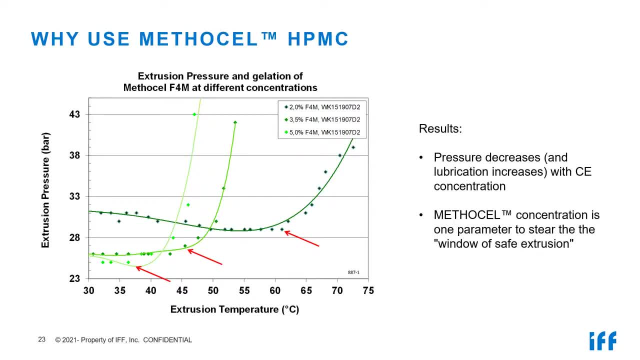 extremely narrow so that nobody reasonable would recommend such a recipe. yeah, there might be reasons to run with a high content of plasticizer for very complex profiles, but then you are forced to extrude very slowly. but we should discuss those topics. there might be reasons, there might be options to save money, to reduce the concentration. 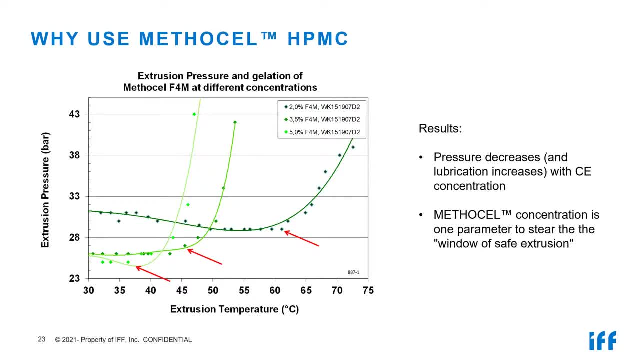 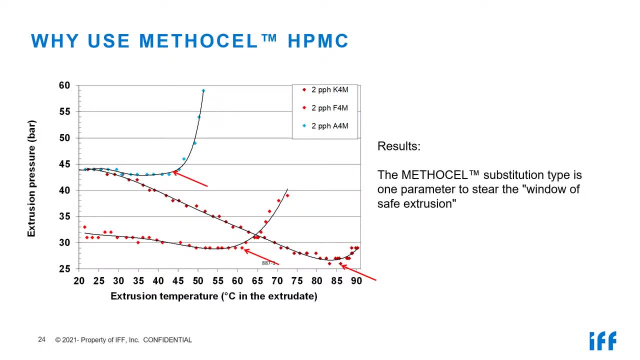 of additives with other solutions. next slide: yes, three other examples. now we are comparing three times same concentration of three different, uh, cellulose eaters. uh, um, here in this graph we are talking not in percent but in pph. sorry, but uh, maybe you are doing the same. pph means parts per hundred weight and this is a. 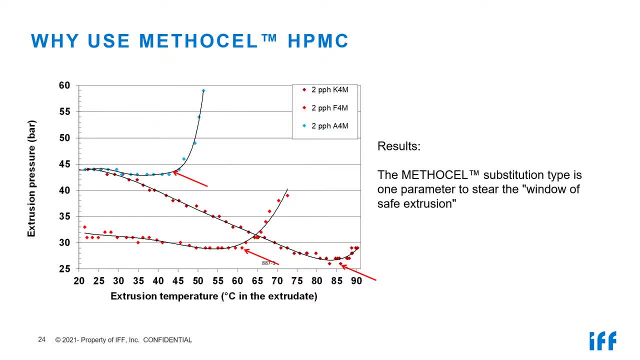 slightly different calculation. so we are calculating parts of cellulose eaters on top of 100 parts of ceramic dry ingredients, and of course then you have still to add the water. here we are comparing three very different behaving cellulose eaters. let's start with a dark red curve. 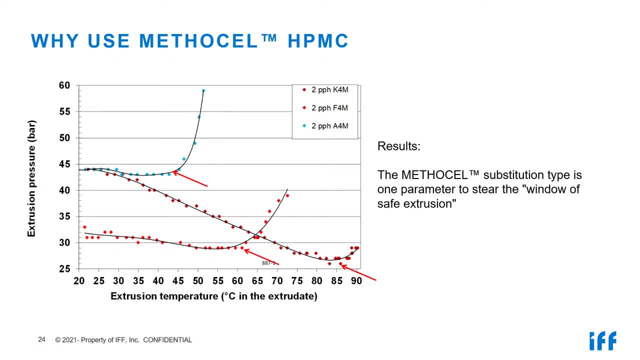 which shows first a long, very linear drop in pressure. because, i said already, if you heat up a polymer solution, the viscosity must drop, but at the end of the scale, somewhere at 80 or 85 centigrade, the extrusion pressure drop stops and there is a rise in temperature. 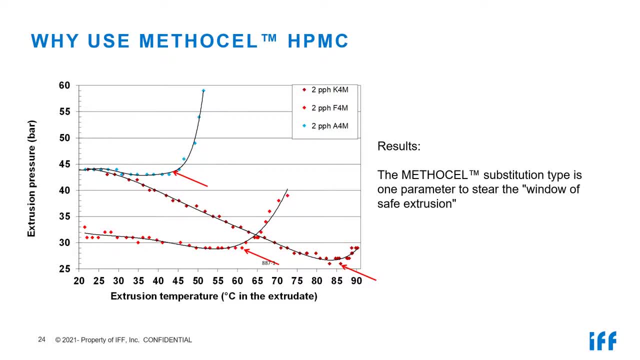 and this is due to the flocculation of the cellulose eater. but this metal cell k chemistry is very well known to lead to very, very high gelation temperatures. so the safe window of operation here is somewhere up to 70 degrees, which is probably good enough for nearly. 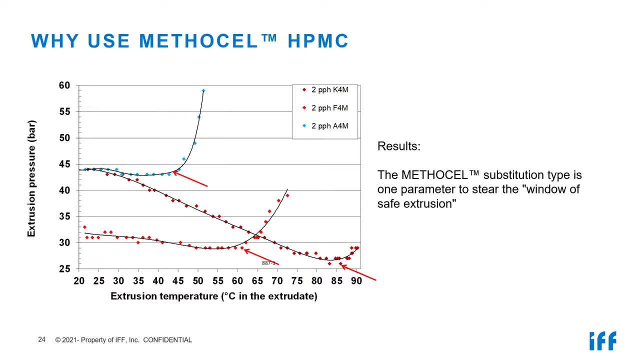 all cases. metal cell f for m is the second example, the other red curve, which shows significantly lower extrusion pressure and also a lower relation temperature, somewhere in the range of 60 degrees. and for special cases we can recommend also the a chemistry, the pure metal celluloses. however they have. 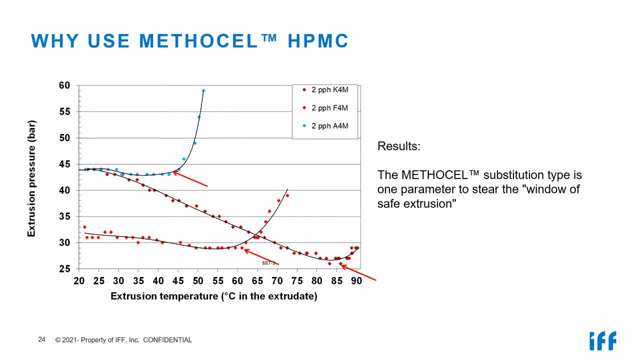 a combination of all disadvantages you have seen so far. they show high extrusion pressure and a very small window of safe operation because the relation temperature here in this case is already at 45 centigrade. however, there are reasons to use it, and it is used in the market, for instance. 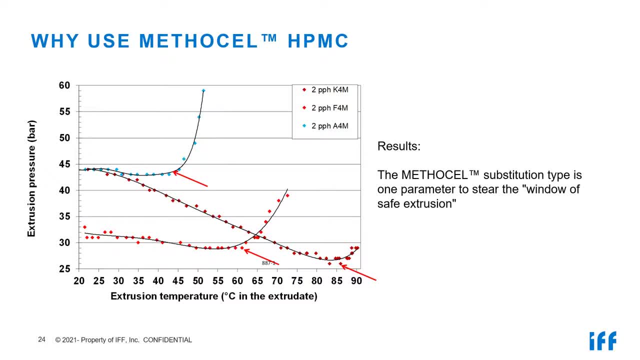 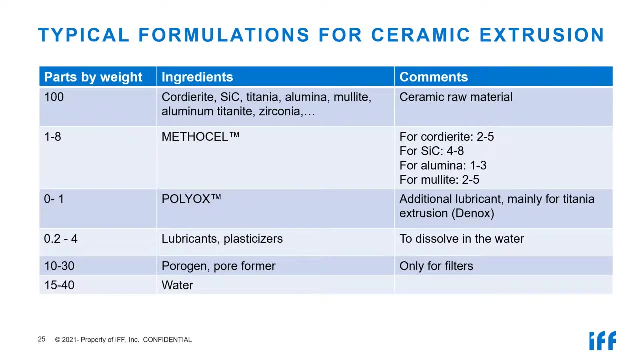 the metal cell. a grades give a wonderful shape retention in complex profiles. this is positive. this is a benefit we should mention. next slide, please. yeah, i would give at the end. i would like to give some typical formulations for ceramic extrusions. you might know it if you run extrusions every day, but if you start just with this topic, 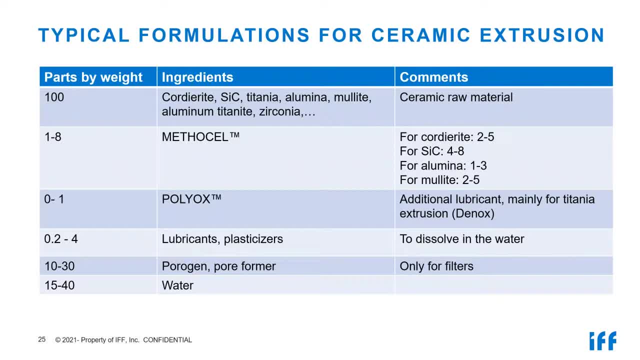 you might be happy to see some guidance. normally you start with 100 parts of ceramic ingredients, whether it is collierite, silicon, carbide, titanium, alumina, whatever- there are many options- and one to eight parts of metal cell and depending on the ceramic raw material, for instance um alumina, you choose a lower content of metal cell. but if you choose, for instance, 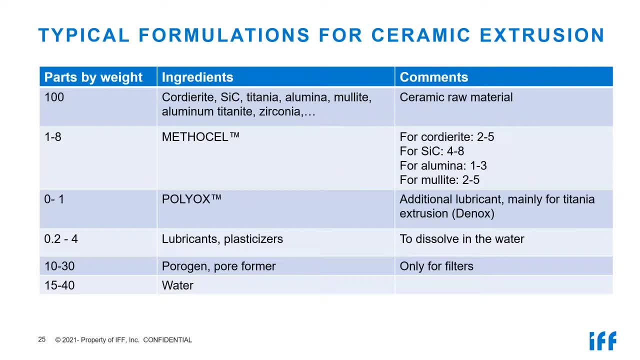 silicon carbide, you need a higher content, four to eight parts per weight. in alumina just one, two, three. an additional lubricant is polyox, which is used nearly in all cases if you extrude alkaline titania honeycombs for denox filters, but it is used also in other extrusion. 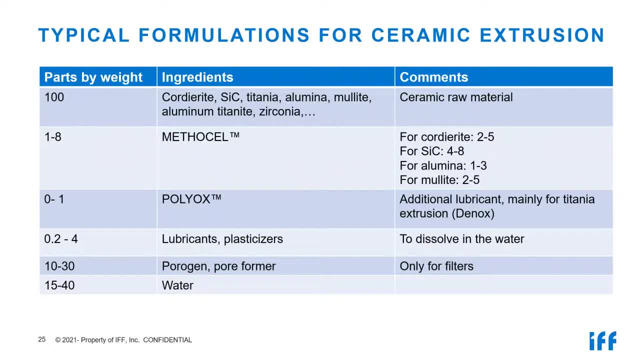 applications and it is an additional lubricant leading to a wonderful plastification of the mess and it has not a big effect on the isolation temperature. further lubricants are used more or less everywhere. you can read a lot of literature about the further lubricants and plasticizers. please use them only as much as needed, because a higher amount always leads to. 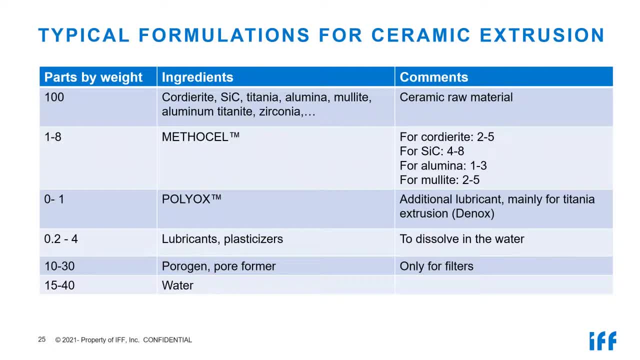 problems in the cohesion of the ceramic particles and also they contribute to a reduced, to a reduced gelation temperature. so always, it's like always a compromise: as much as needed, but not more. and if you extrude filters, then it might be um worth to think about more formats. there are many performers in the market. 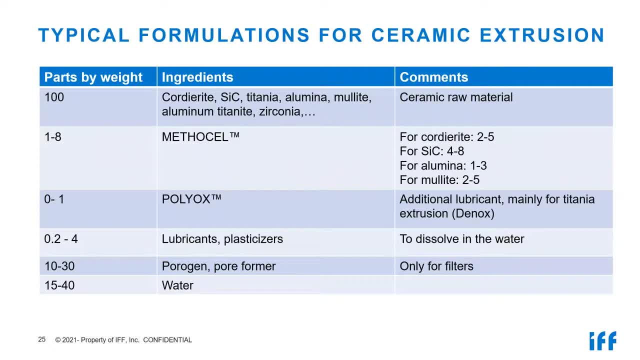 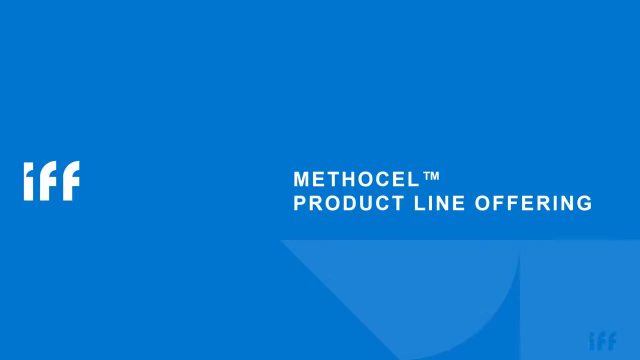 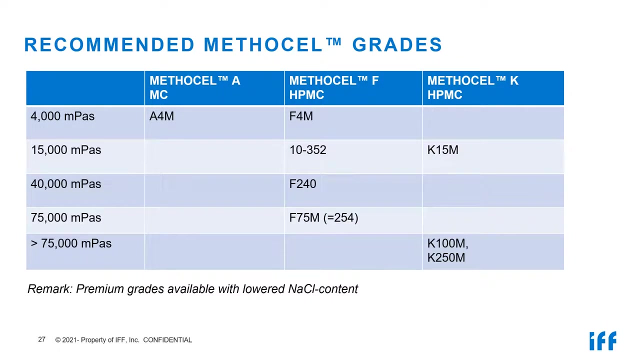 and, of course, at the end you need a certain amount of water to get a stiffy paste and the amount depends, of course, on several parameters, like the particle size distribution, like the surface of the ceramic particles and some other parameters. next slide, our product line, yes, next slide, please. um, we have a huge product line. uh, we do not recommend everything. 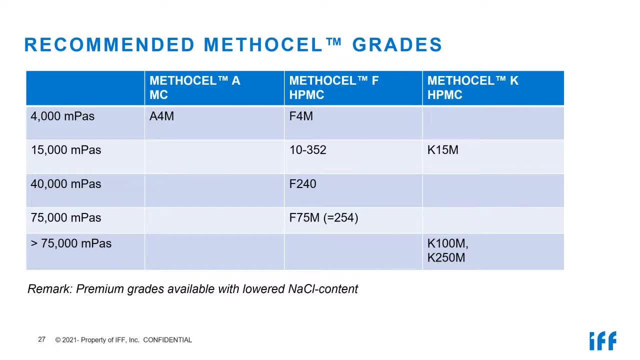 for ceramics. here is just a selection of the most- uh, let's say most- famous materials. here we are presenting three metal cell classes: the metal cell a, the pure mc and metal cell f and k classes, all having different viscosities starting from four thousand up to um 75 000 and even higher. 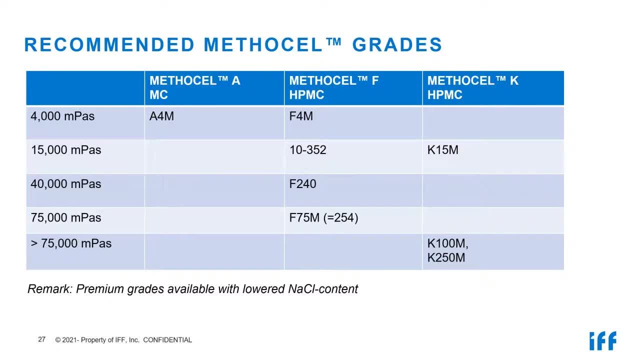 everything is possible, but not everything is possible, but not everything is always reasonable. so, um, there are many reasons to use this or that formulation, and this is, of course, subjected to an individual discussion. also, i should mention, we have still some special grades for special purposes and special requirements. um, we can. 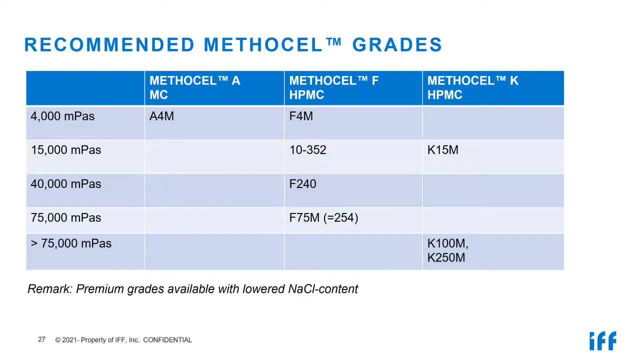 discuss this on demand and it's worth to mention. we have also premium grades because we are big supplier in the pharmaceutical industry. we have also premium grades because we are big supplier in the pharmaceutical industry. premium grades contain: contain um significantly reduced sodium chloride content. this might be. 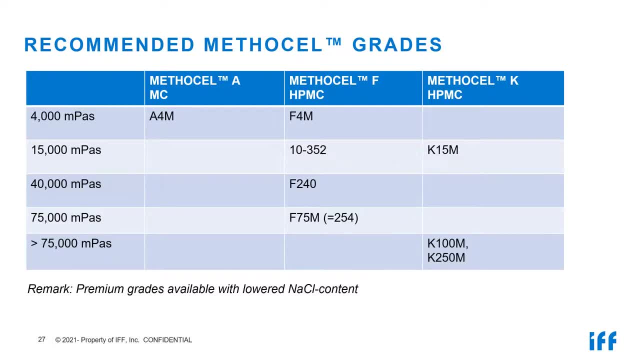 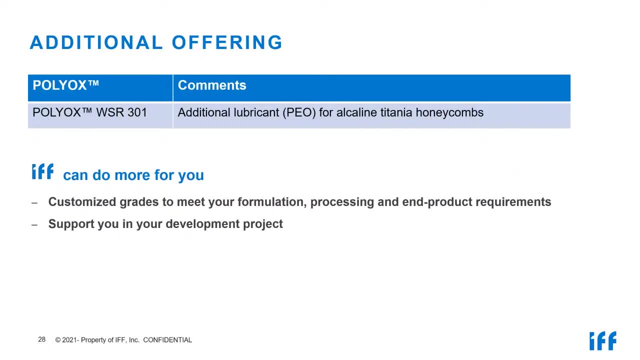 interesting. if you want to extrude catalysts, next slide, please. yeah, here still mentions the polyox grade wsr301. this is a polyethylene oxide with a molecular weight of 4 million. this is our multi-purpose grade. if you like, as additional lubricant, yeah, we, um, we are open for a discussion. um, if you like, we can do this offline. 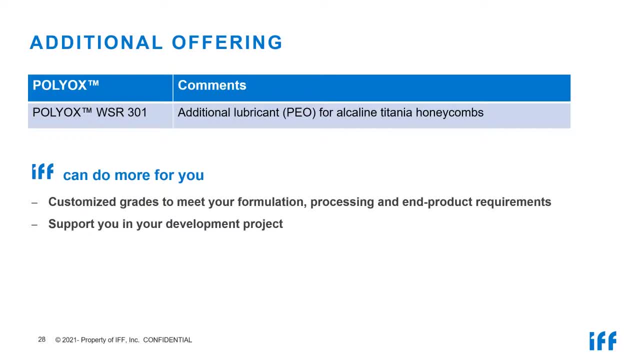 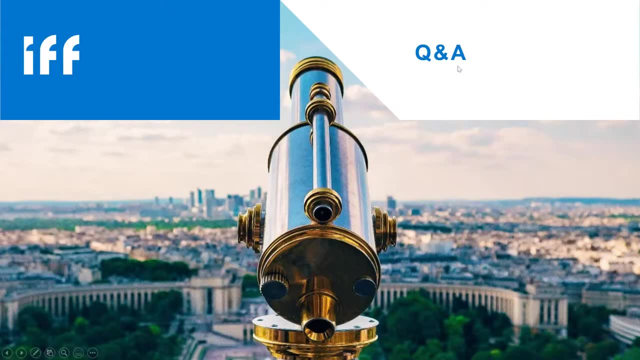 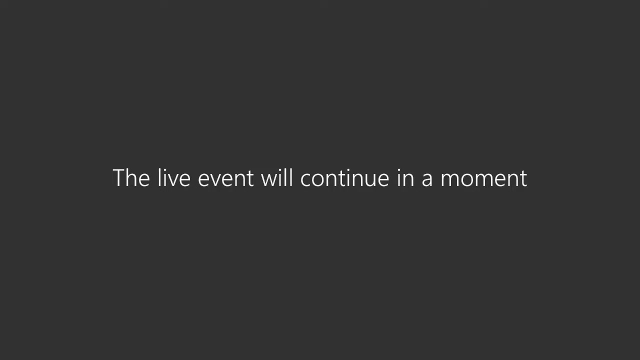 you have the address of camp point. we have customized some customized grades and happy to receive your feedback. and with this i would like to finish and open the question and answer session. thank you, roland. let me check and see questions we have here. looks like we have a couple coming in one second here. 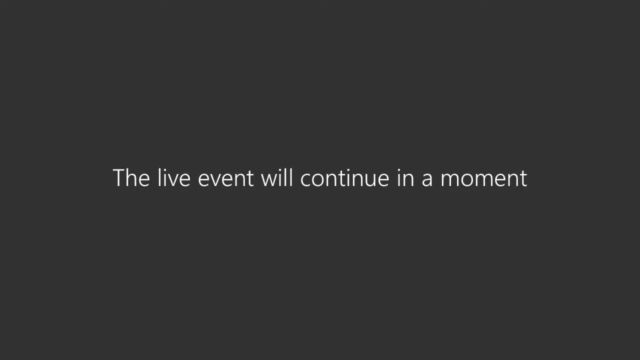 i also think a lot of people were saying here: thanks for your questions. again, if you have a hard time finding the question and answer, live Q&A box if it's in the top right of your window there a chat bubble with a question mark in the middle. so if you'd like to submit a question, feel free to do so now. 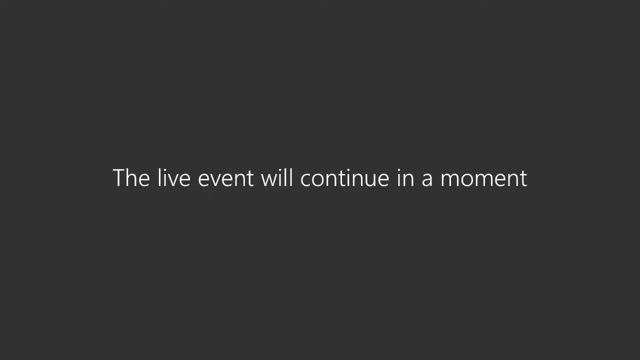 all right, looks like we have one question here, Roland. how do the different met the cell classes AEF, K and J differ in regards of their content of substituents? yeah, thank you. I remember there was one slide in the slide deck showing these boxes. these boxes represents specification windows, the specification window of each. 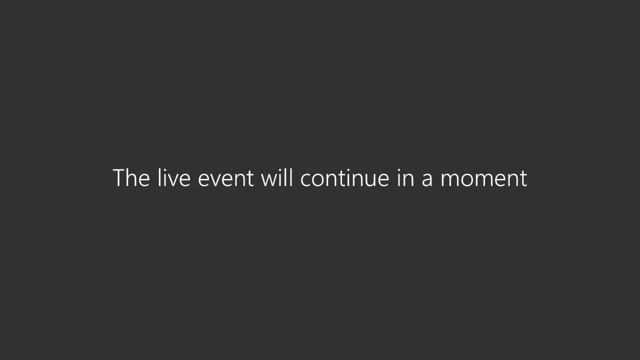 product class. however, the scales- the X and the y-axis, are given in percents. these percents are coming historically from the definition in the pharmaceutical industry, so they are part of the pharmacopoeias of United States, of Europe and Japan and many other countries, and there is still, I should 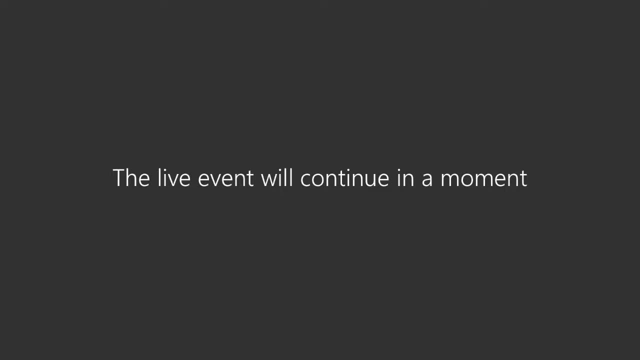 mention, there is still a scientific definition which is different. they are not calculating the methylation and hydroxypopulation degree in percent by weight, but in in in in numbers. so for instance, they consider a single glycolic unit. so in this case every glucose unit has three hydroxyl. 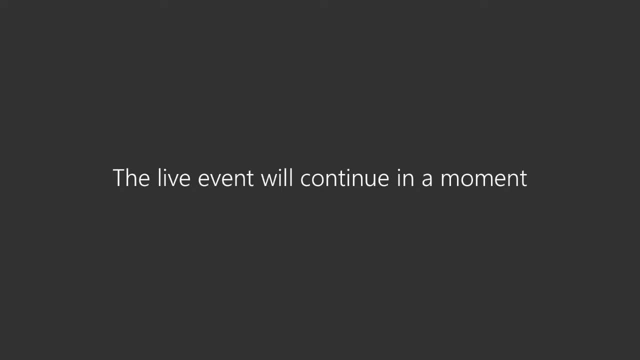 groups. so in maximum you can replace three. so this is a so-called DS substitution degree or the modulation degree. you can never add more than three metal groups to the hydroxyl groups to the hydroxyl groups. so the maximum is three. in the case of hydroxyl population it is a little bit different because the with propylene oxide can lead to small side chains, so one propylene oxide molecule can react several times. so with each other, no, not with itself, but with other molecules, leading to two, three, four, five or six or even more um smaller hydroxy propyl groups, and they 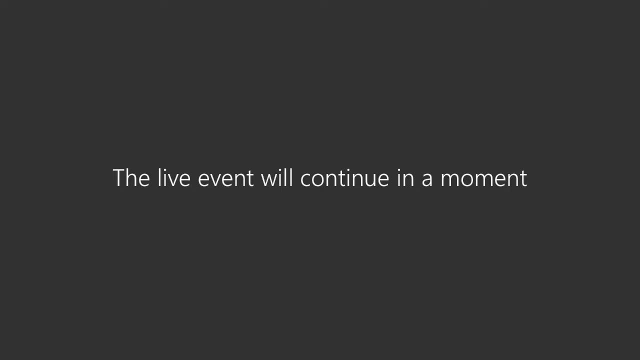 lead to a little chain. so theoretically the substitution of the hydroxy propyl groups could be much higher than three. but of course this is a question how to steer the reaction, how much reactants we enter into the reactor and we have some. we have a lot of control. 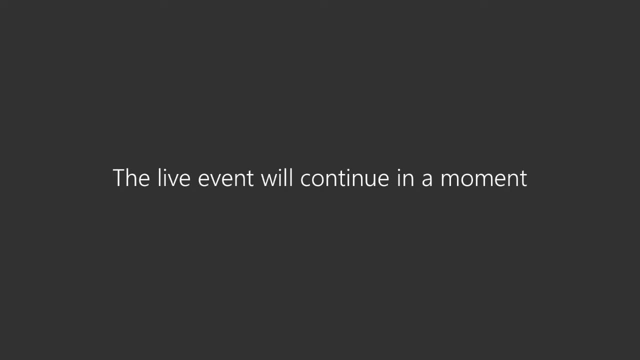 of course on on the reaction chemistry. so we can clearly stay in this windows as we defined them, and they are also mentioned in the specification, and if you receive the analytical certificate, then you know where exactly your batch is located in this box. all right, thank you, uh. question here, uh, from. 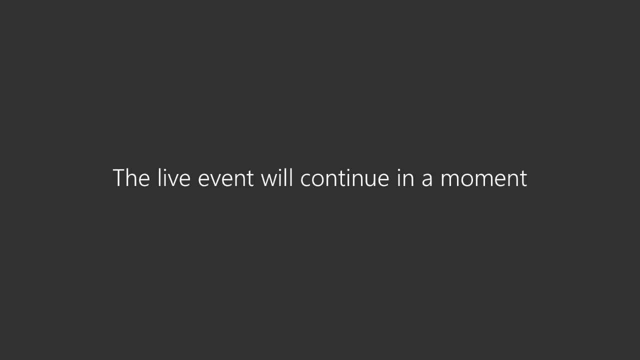 amir, is hydrating the hpmc prior to mixing with other powders an option, or should it be dry mixed with other powders followed by addition of water? ah, the most efficient way is to start with the dry mix. dry mix between the ceramic ingredients. 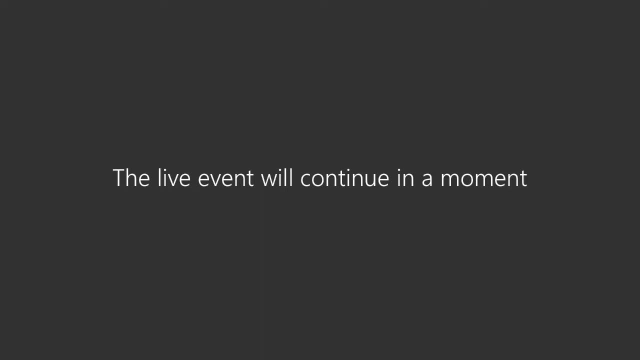 and the cellulose eater, because once you have water in the system, you get a high viscous material and a stiffy material, and to add another ingredient into a stiff material is much more complex than to make a homogeneous powder mix. by the way, once you have this homogeneous powder mix, 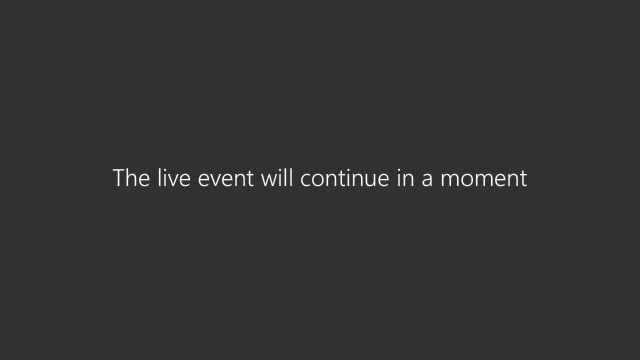 you should not pump the water into the mix, because then you do not. you will never get an even distribution of water into your ceramic mass. you will always have an uneven distribution of water. we have made measurements and the distribution differences can be more than one percent, and one percent more volume or less volume is already a reason for crack formation. 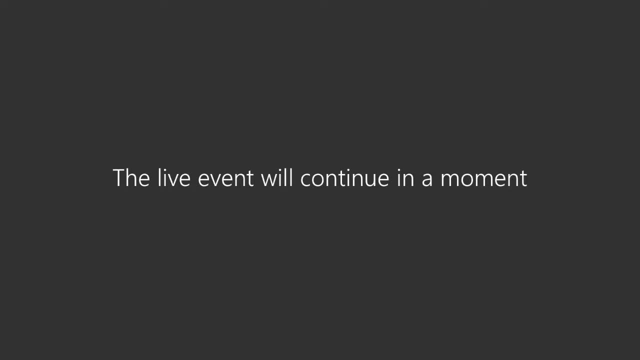 when you dry or when you sinter. so this is very important: not to pump, but to spray the water into the bridge. and it is easily done. yeah, a spray nozzle costs you ten dollars, maybe twenty, but this is really a not not an issue, but you need to guarantee that the water is homogeneously distributed. 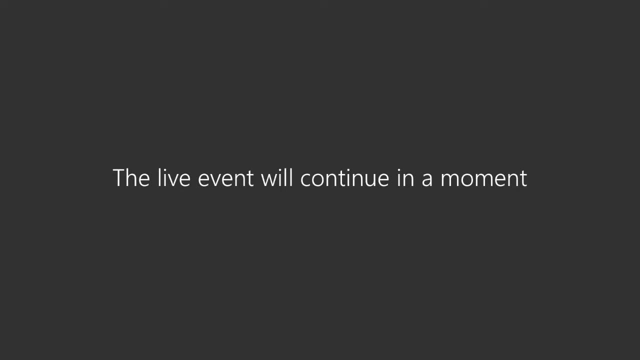 over the whole batch. everything else leads to very complex processing or ten hours of needing time, and this is a nightmare. it's reducing your capacity in the plant and it is leading to lots of abrasion, costs you high energy and produces potentially also off speak thanks. next question. 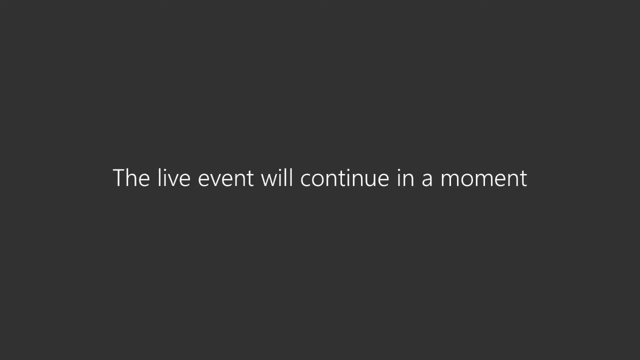 here is: how does shape retention correlate with the different chemistries? ah yeah, very interesting. so this is obviously a question from somebody making a whole profile. as this is my assumption, i can give you a rule of thumb: um, to give very nice and good and stable shape retentions, i would 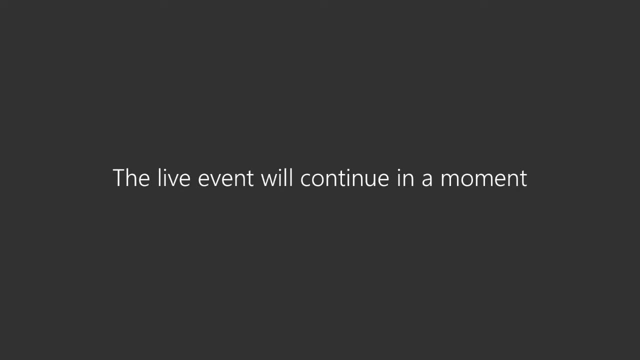 first. my first choice would be also always a metal cell k chemistry. if you do not have a wonderful control of temperature, if you have a very good control of temperature in your plant, you can also choose metal cell a. this works. but you remember the slides and you will receive them definitely. 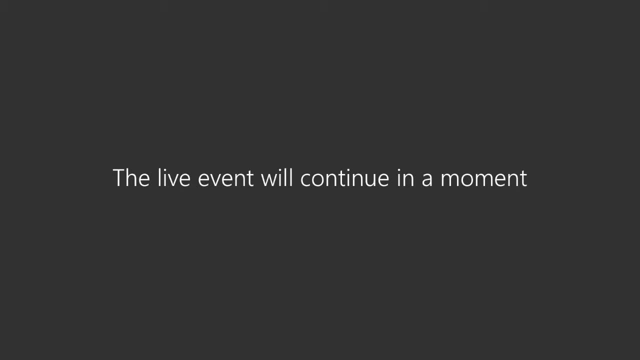 um. metal cell a has a very small window of safe, safe operation. so you must have a very nice temperature control on plant um, um on the plant scale um. it's it's worth to mention that the paste which you get with the metal cell k? um behaves a little bit different from a paste you get with the 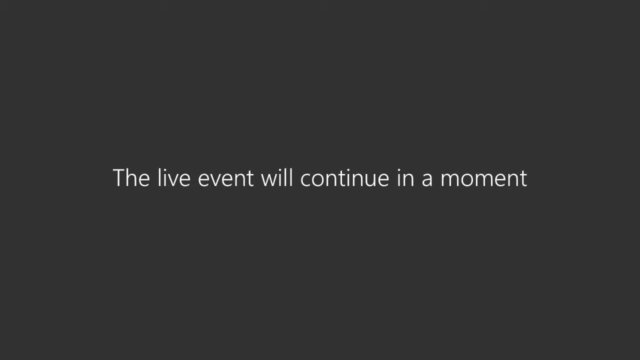 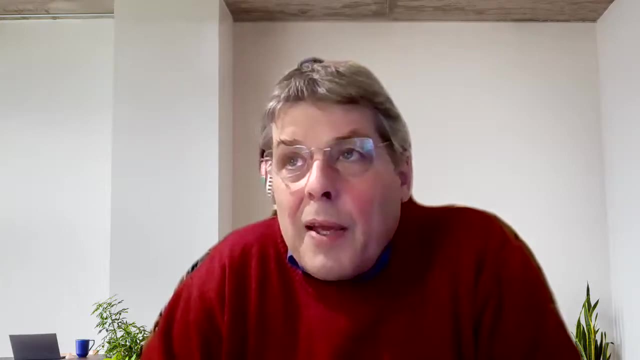 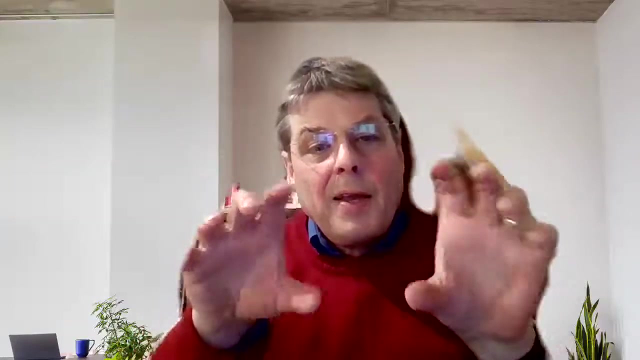 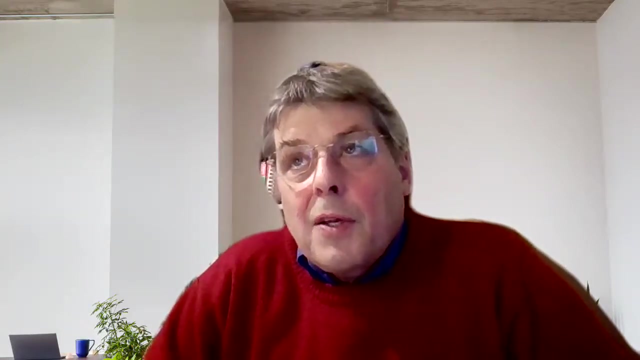 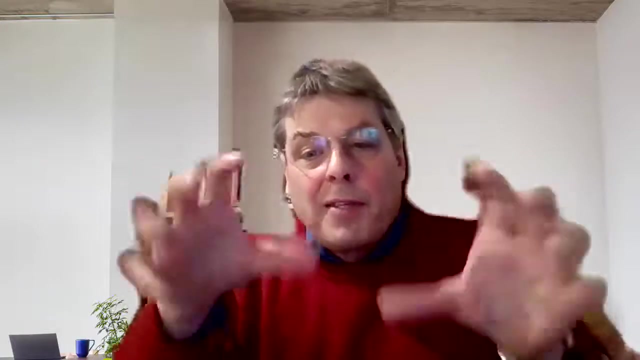 metal cell k, cell f um. so for instance, the paste ductility um with the metal cell k type is um. it is stiffer and if you bend the profile in your hands, uh, you will see easily a crack formation. so the sensitivity to um it's more a rigid profile where the profile with metal cell f is more flexible. 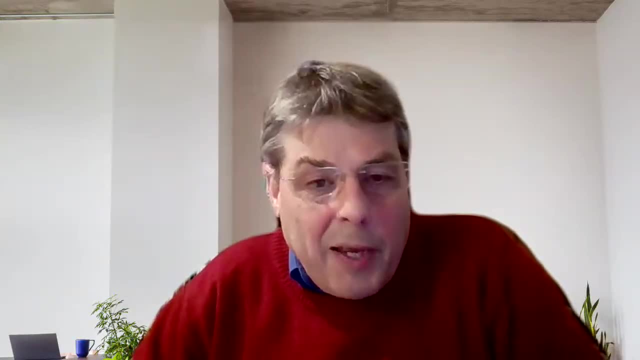 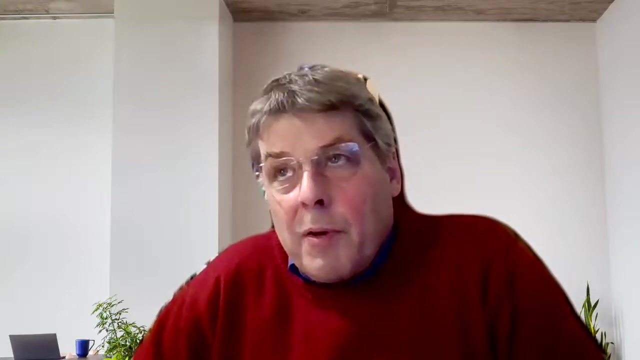 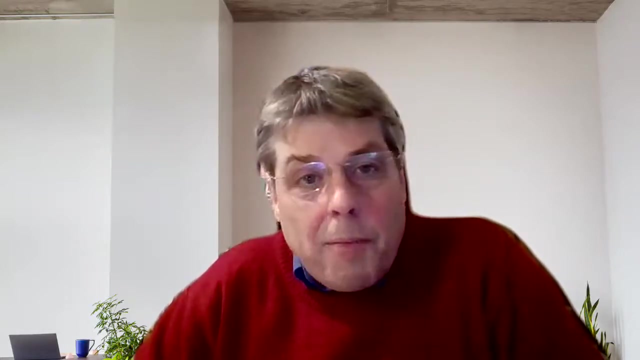 yeah it, you can bend it a little bit more before you can see the first crack. this is, of course, a very qualitative test, but you can easily make it, even on a lab scale and check the profiles. um, you can also develop a qualitative test to check the shape retention if you make a three-point bending test. if you like, we can. 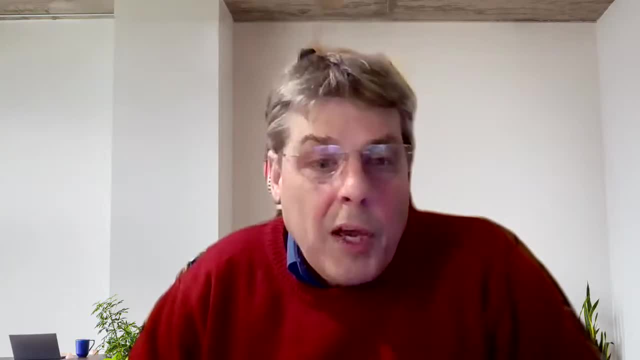 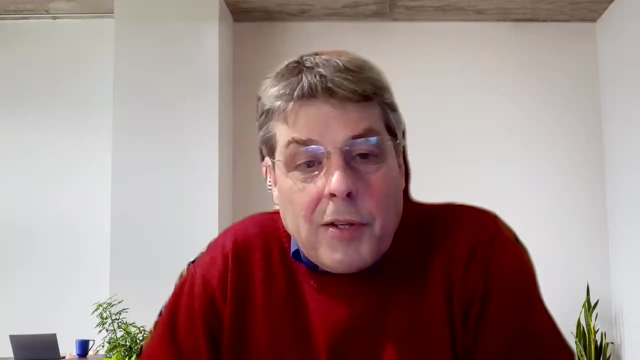 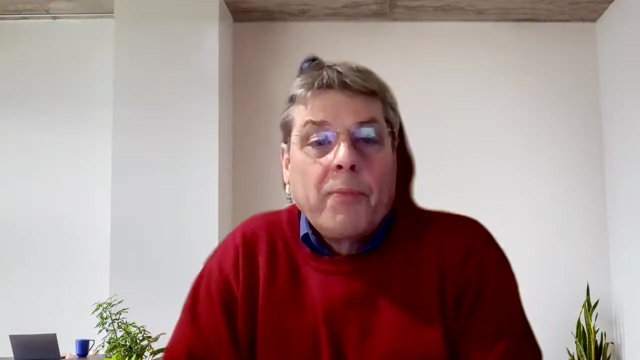 discuss details offline. we have developed a method which we routinely use. it's a very simple test, a three-point bending test with a fresh extruded profile, and this gives the first indication in the direction where to go. but you should do it with a full profile, never with a hollow profile. 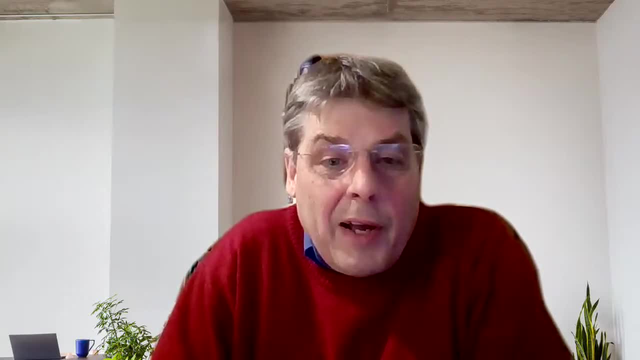 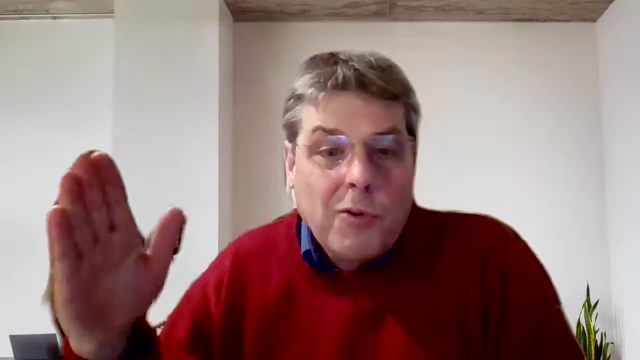 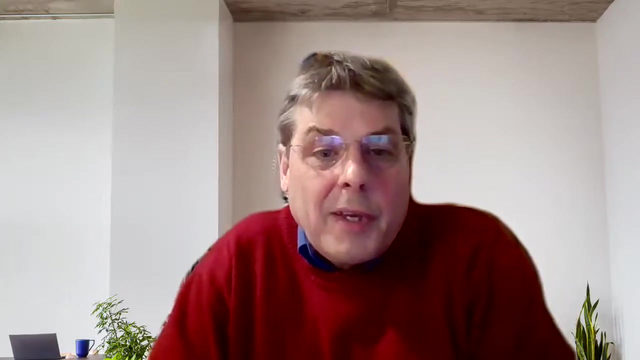 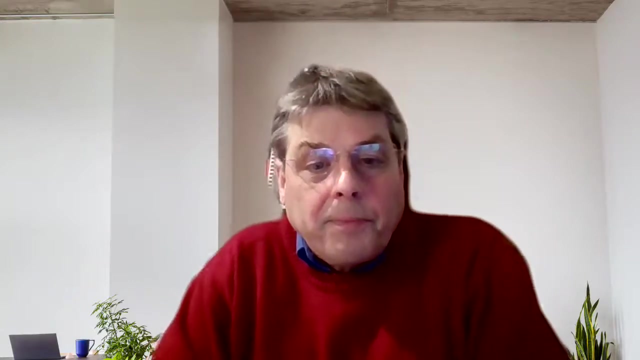 you because hollow profiles are drying so fast they are losing water during the measurement and you get a permanent deviation of the measurement during the test run. so you need necessarily a full profile just to see the differences in the shape retention data in the different recipes. great, thank you. so we have another question here. uh, can i use the? 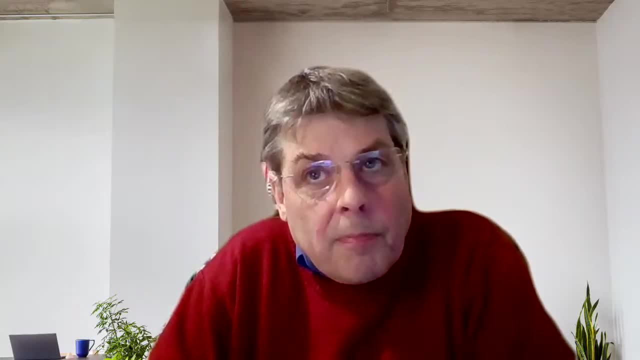 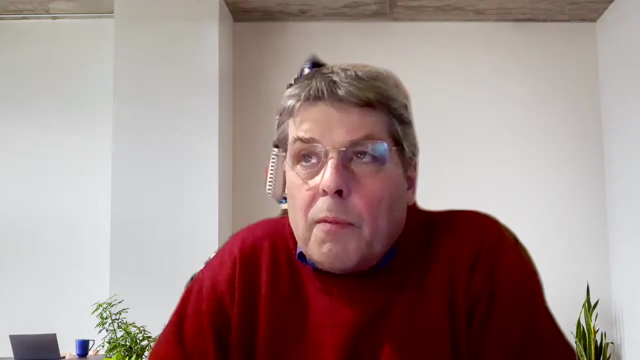 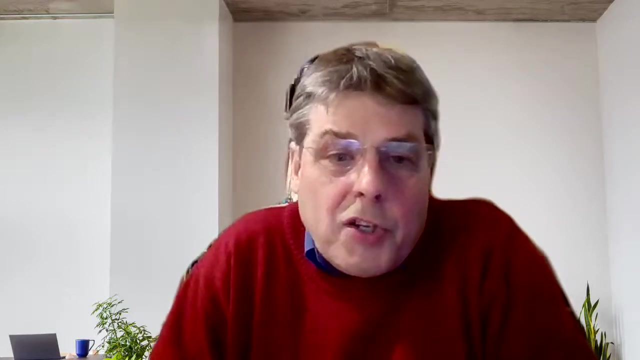 combination of a and k types and then, in addition, is there any plasticity data of paste made with type a and type k? yes, combinations are possible. um, this is not unusual and i would not expect a major issue, of course. um the isolation temperature of a combination of a and k. 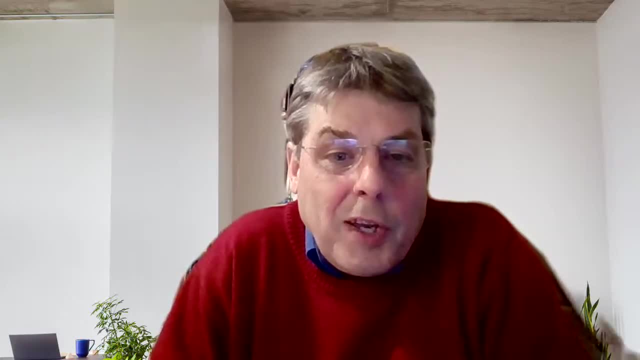 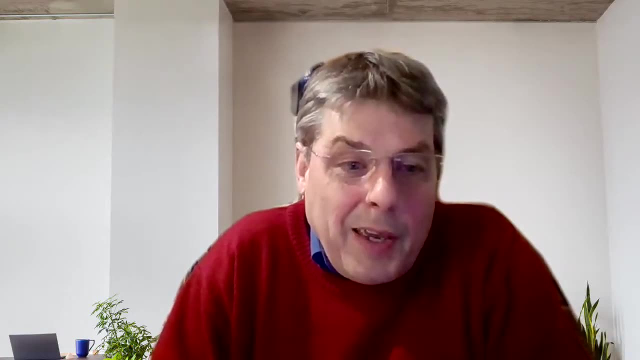 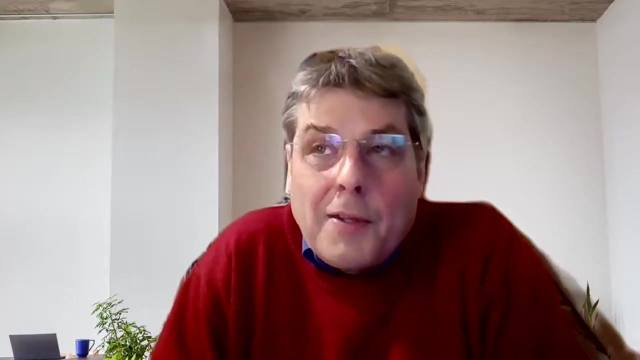 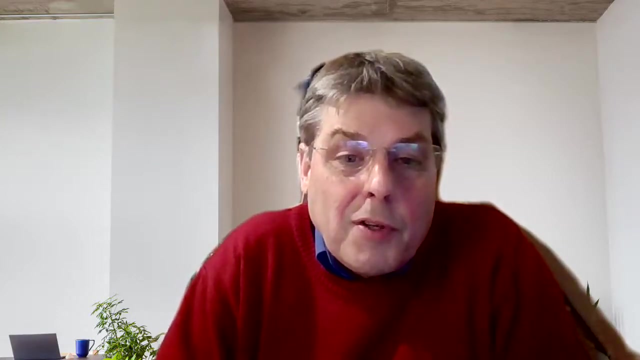 will not be somewhere in the middle between the two extremes, but the? a molecules will, will gelate there where the? a chemistry relates and the k molecules will relate where the k molecules relate. so this means the total mix will show will require also a very good temperature control. then it is possible. 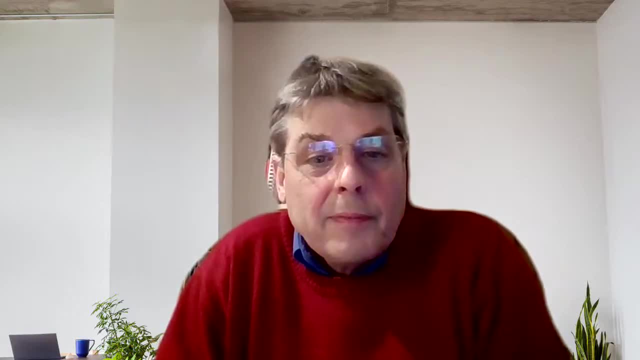 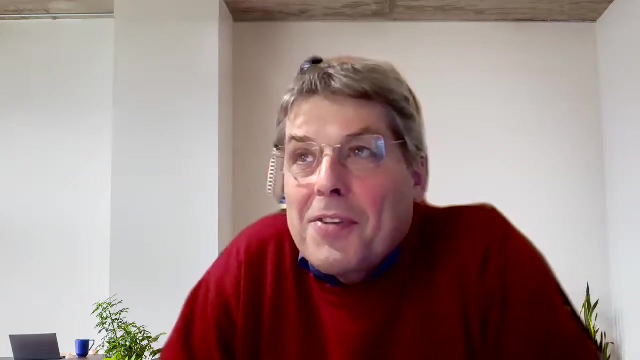 let me just see if you have any new questions coming in here. looks like one other question here. uh, you said earlier, the methyl acts as a binder and thickener. do you have grades available where there's only binding or only thickening properties? ah aha, this is a very nice question, um. 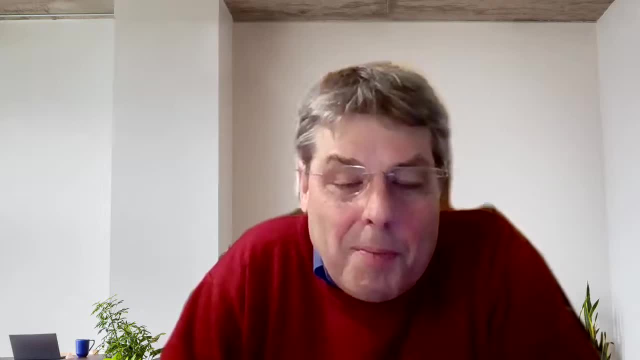 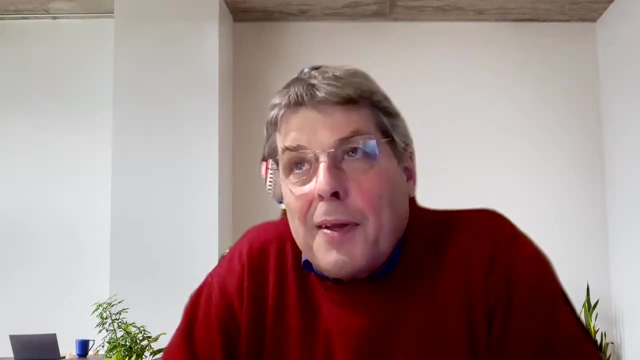 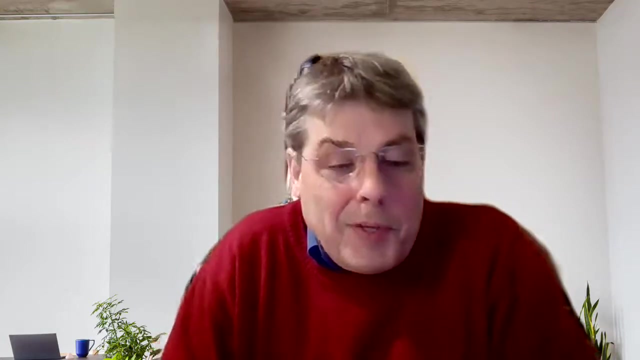 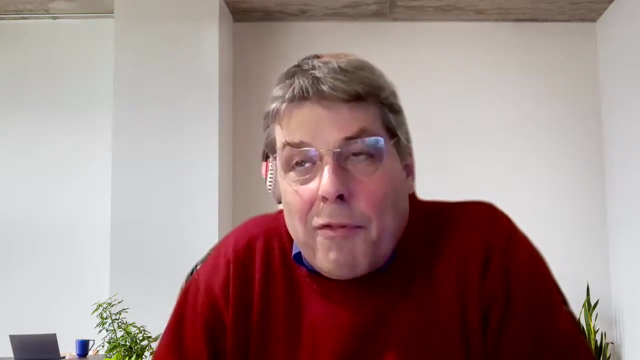 maybe i said: uh, you said earlier, the methyl cell is a multi-purpose additive, so you have many properties unified in one product. um, now the question leads me to the conclusion. maybe somebody needs something which is just a binder or just a thickener. this is not possible, but you have another option you can. let's. 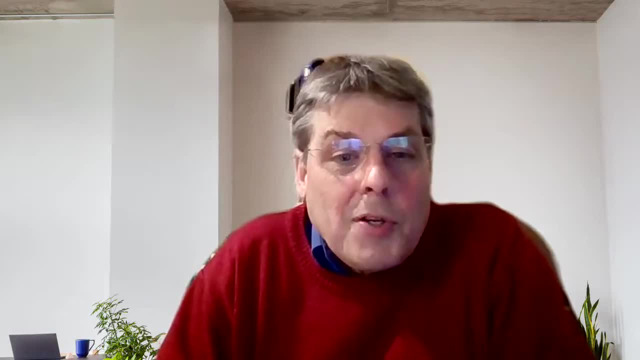 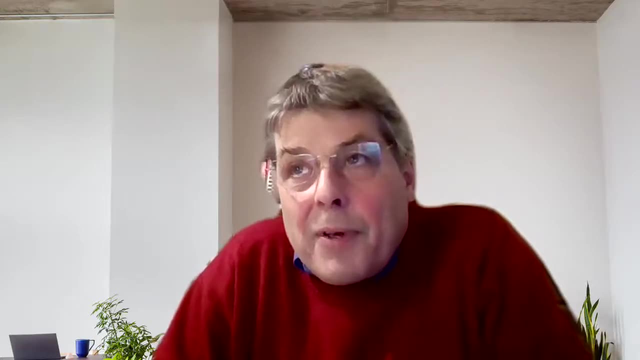 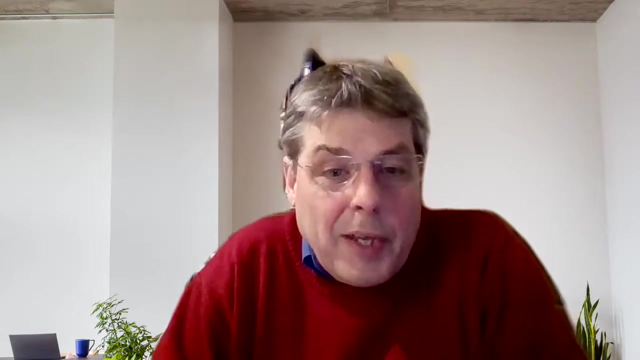 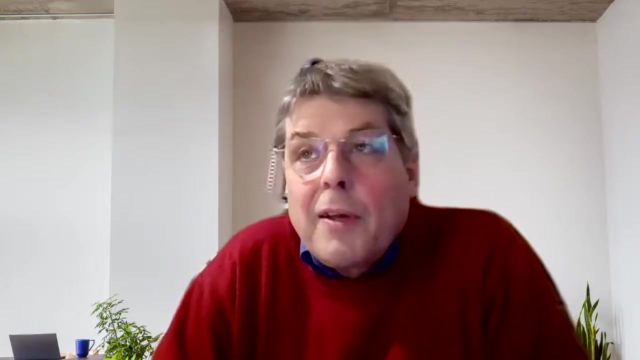 say: um, you have. we have grades available which where the thickening effect is more dominating, and other grades where the binding effect is more dominating. obviously is that high viscous materials show a very strong thickening effect, whereas the low viscous materials do not show a significant thickening effect. 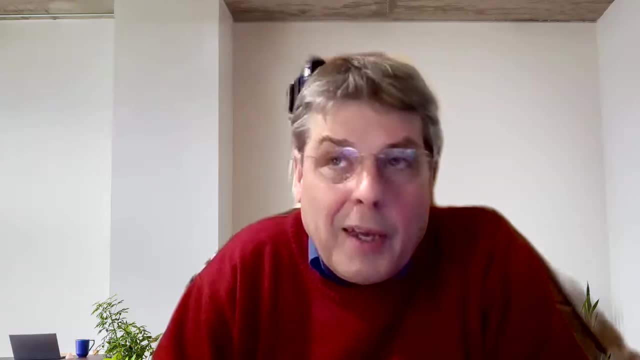 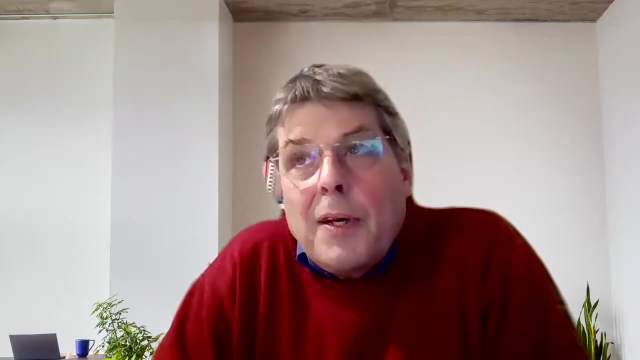 only a little thickening effect, but you cannot reduce the thickening effect down to zero. um, in both cases they show a binding effect. so, um, you can, let's say, modify the relation between binding and thickening, but you cannot reduce the thickening effect to zero and also not the binding. 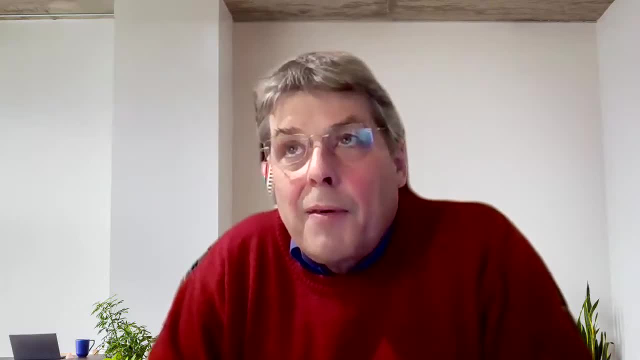 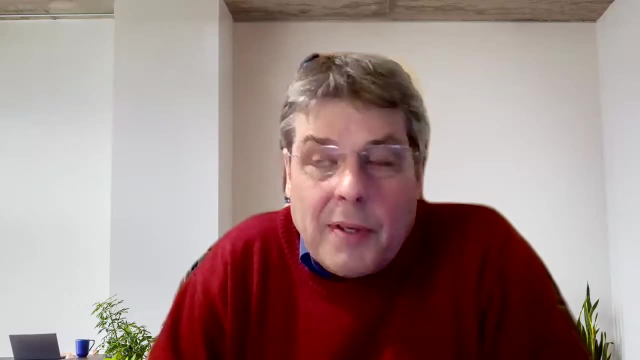 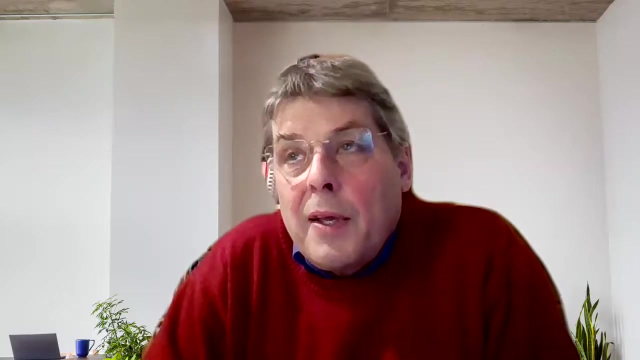 effect down to zero. if you make, let's say if you formulate a batch um, one batch with very high viscous cellulose eta and the same batch with the same amount of a low viscous cellulose eta. you have strictly reduced your paste viscosity, but you have still the same binding properties. 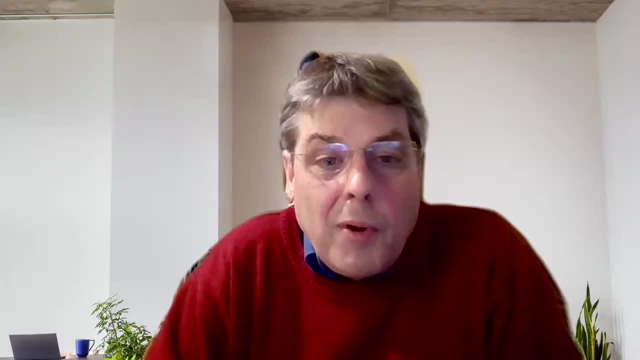 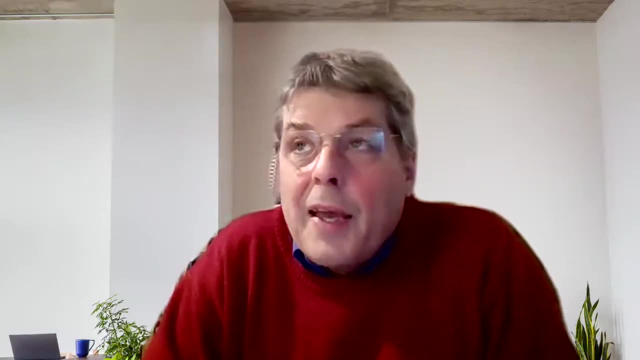 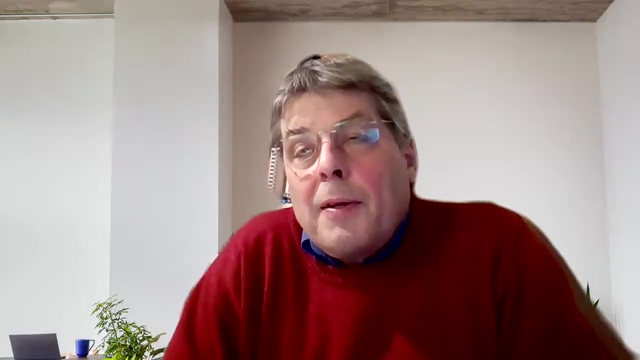 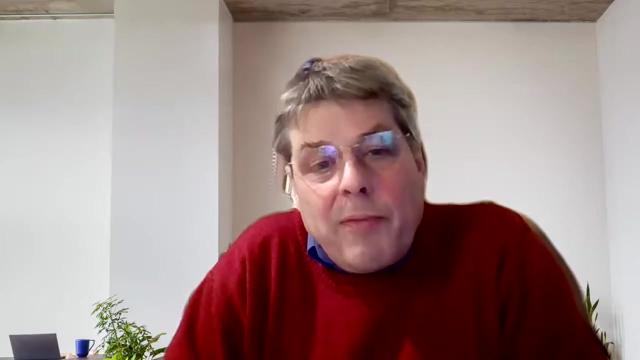 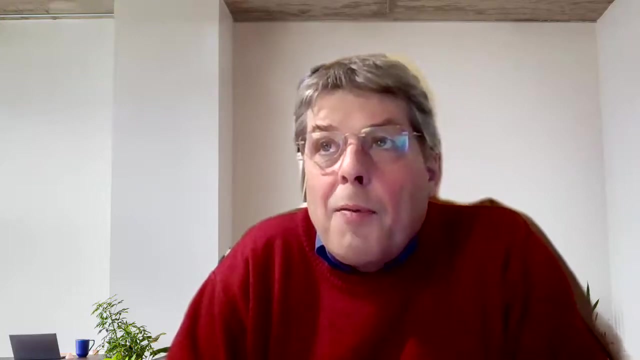 binding comes just from the cellulose eta molecules surrounding the ceramic particles. this remains the same, just the viscosity at the end is different. um, but um, it's very important, always from a more fixed perspective, um, first to mention that it might be possible to make formulations with very low viscous cellulose ethas. 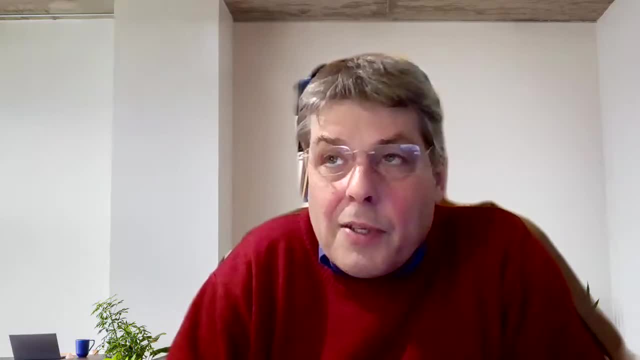 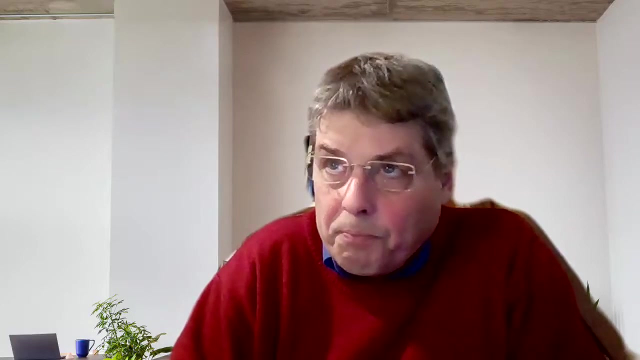 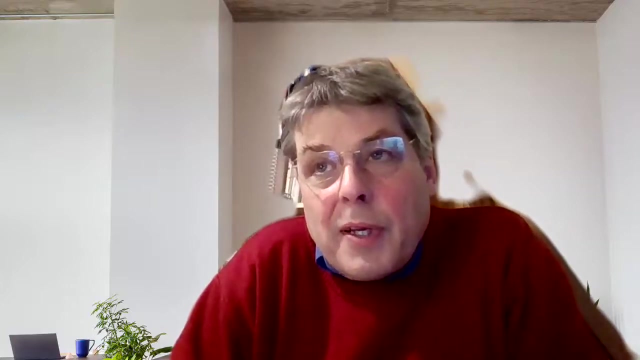 where you have a much more newtonian rheology. um, because this you do not have so many long chain molecules but very short chains. um, if you do not, the newtonian properties are dominating. this is a very different extrusion process, very, very stable. but you should please consider that also the water retention capability is a function. of the viscosity, and once you reduce the viscosity in a too high extent then you might lose too much water retention and this is worth to test. somewhere there will be a limit. so, like always, there is an optimum somewhere and you must find it. but you can try, but definitely i would not. 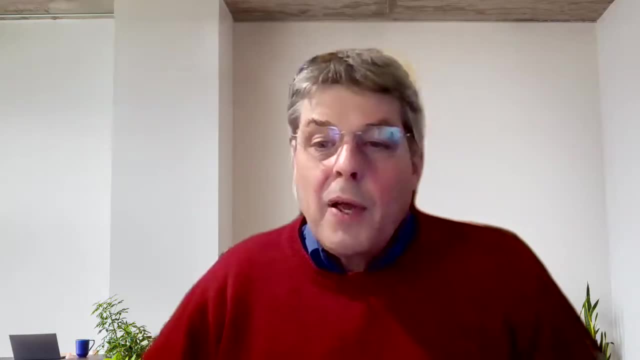 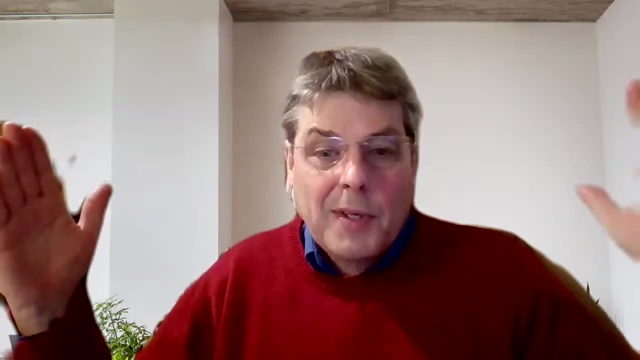 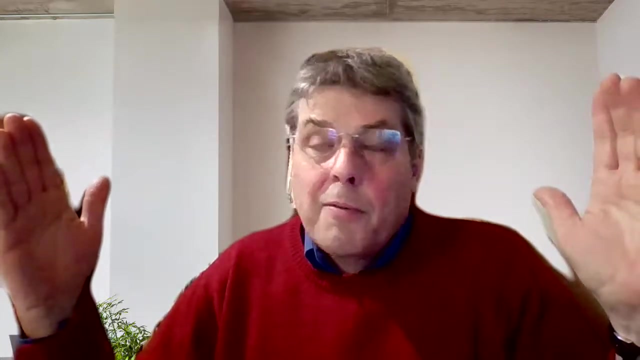 choose a very, very low viscous cellulose eater. you know our metal cell product portfolio ranges over five magnitudes in viscosity. the lowest um viscosities which are regularly sold uh is for instance metal cell k3. three millipascal seconds in two percent and the upper 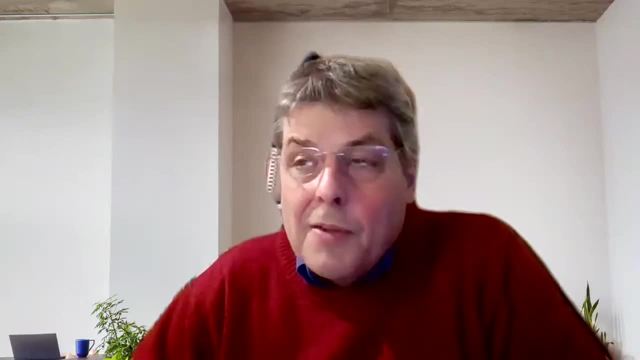 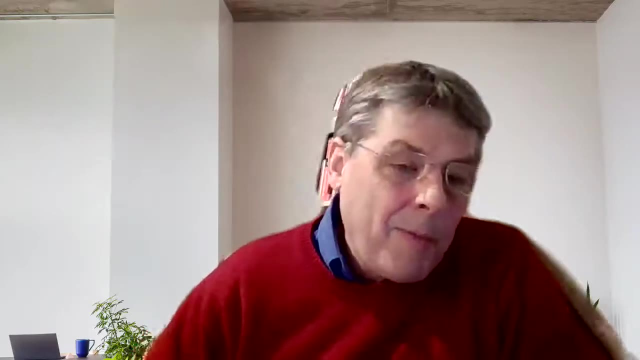 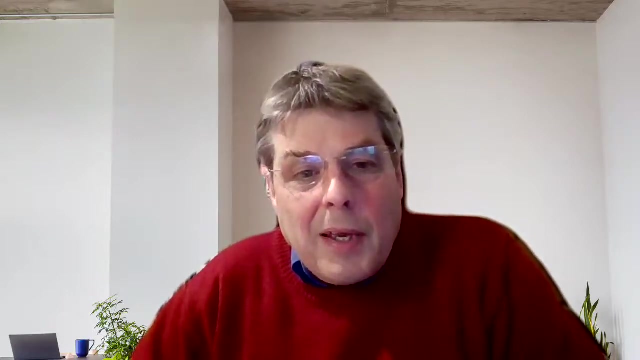 end is somewhere in the range of 100, 100, 000. there is one grade with 250 000.. so these are five magnitudes and of course the properties from one end to the other are changing significantly. um, but it's possible to do this, yes, and it might have some benefits in special recipes. but 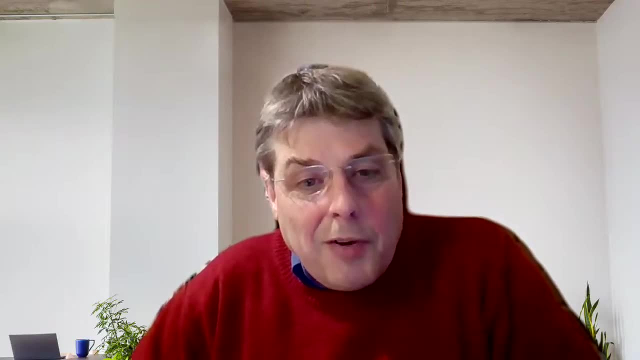 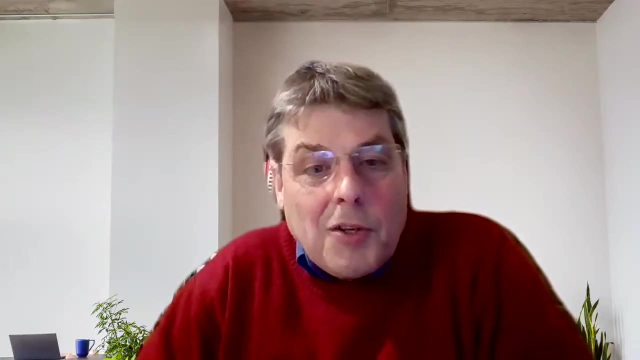 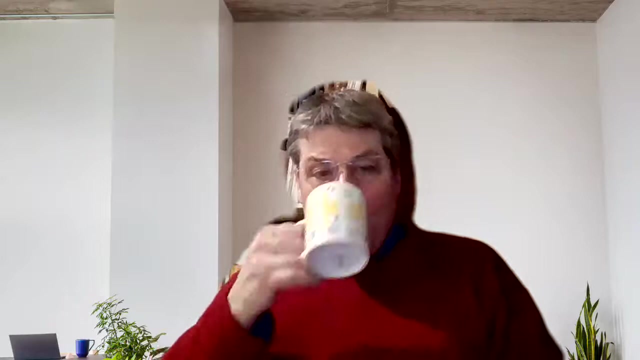 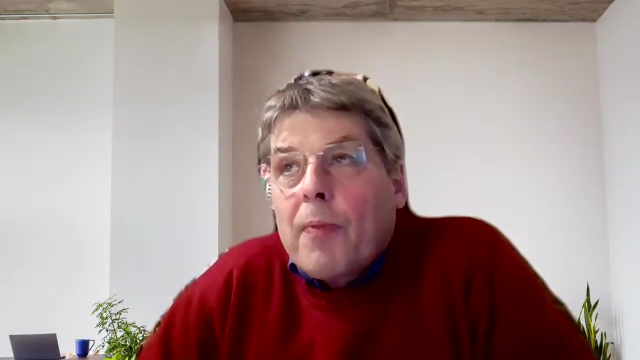 please make first checks that your machinery will not get defects because of the water retention which decreases too much. great, looks like we have time for one last question here. uh, is there a general correlation between extrusion speed and pressure when extruding pace containing methazole? yes, as higher the pressure and 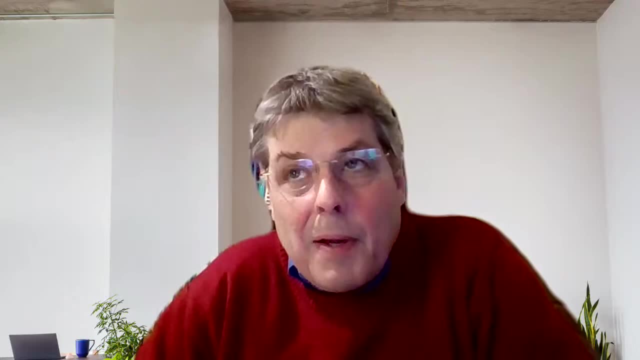 as high as the speed can be much, but not in all cases must be. it is a question of the rheology and i remember, um, we have made trials, uh, 12 years ago, with special rheologies of the paste where we could show that we could increase, increase the. 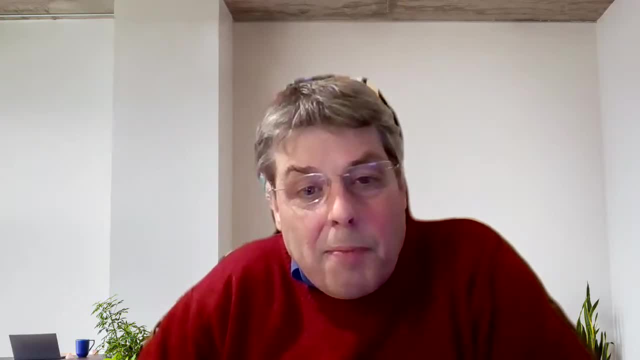 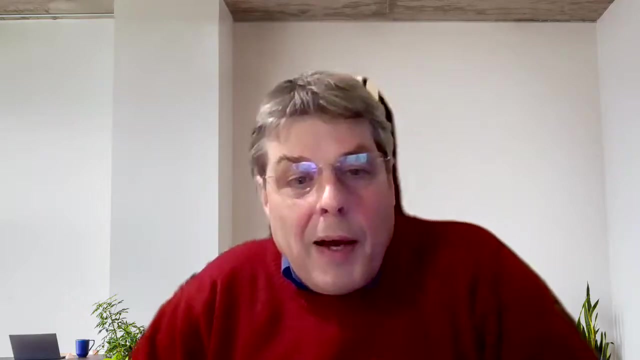 resulting extrusion speed, so the speed in meters per second coming out of the machine. we could increase the extrusion speed by 250 percent and at the same time reducing the extrusion pressure. this was a very significant effect and has rheological reasons. there are some tricks behind. 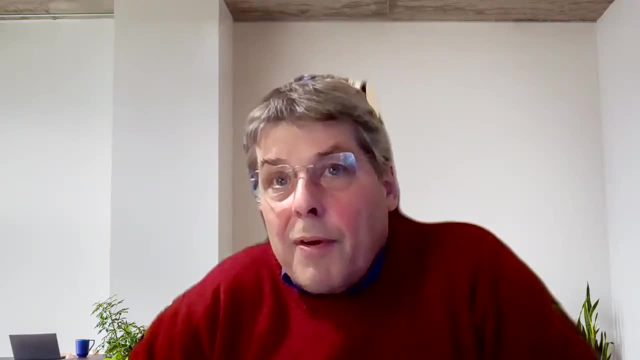 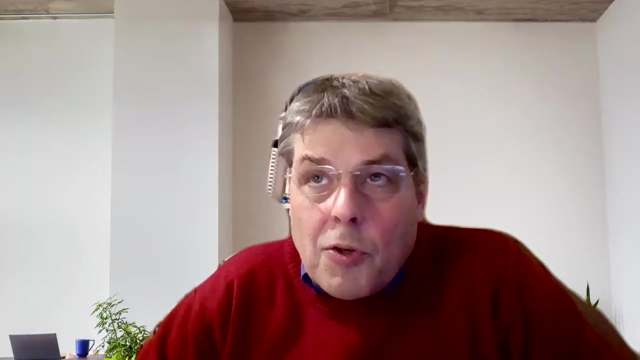 and the background knowledge you should have. uh, i, i couldn't present this because then, uh, um, i had to add 50 more slides. uh, the background effect is, um, the drop of very high, the strong drop in viscosity, of very high viscous materials under extremely high shear. they are dropping more than normal viscous materials and if you run an extrusion. 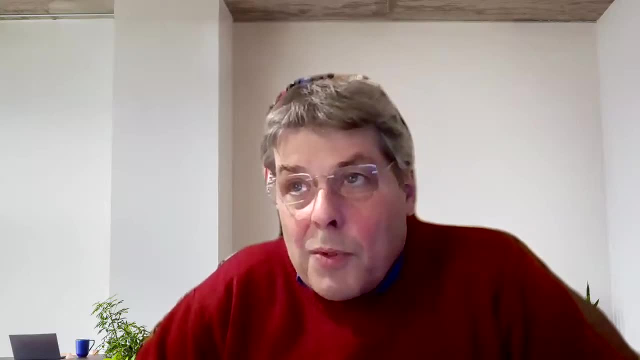 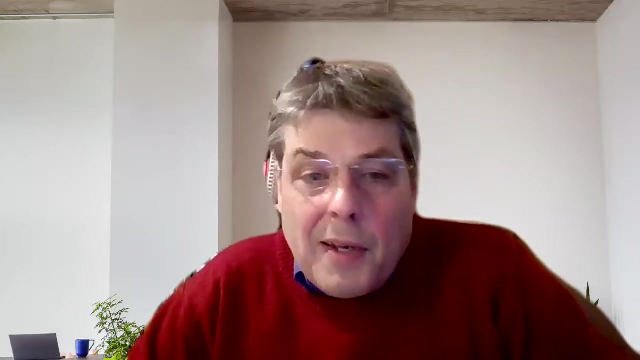 process with a complex die and you use, for instance, k100m or k250m um in a very low concentration, you get a extremely shearsening process and you can extrude with very high speeds um we had. we made a comparison test with f4m, which is, let's say, the blockbuster everywhere and the standard which we are selling. 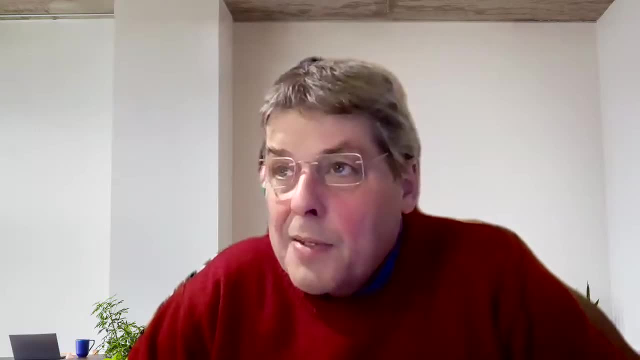 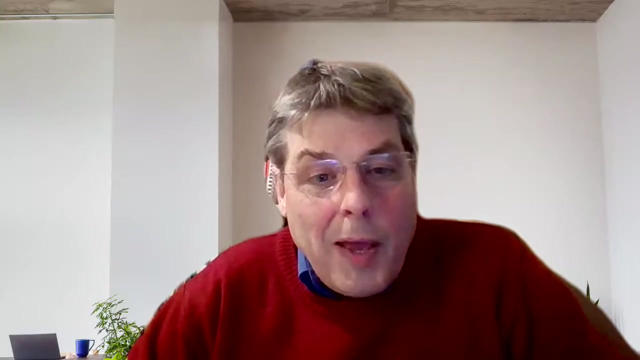 uh in all continents, to many, many customers, and the difference was 250 resulting speed at a lower pressure. so it's not always uh necessary to. it's not always necessary to have double pressure if you ex wants to extrude faster. this is a real cost saving. lower pressure means lower energy costs. yeah, but we can discuss offline if you like.